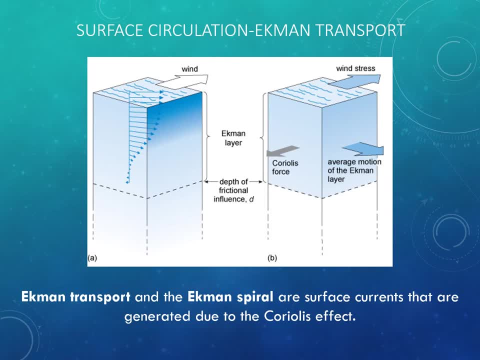 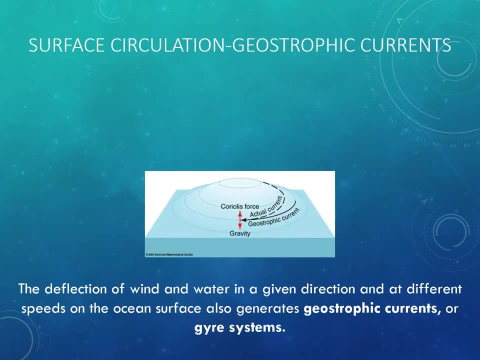 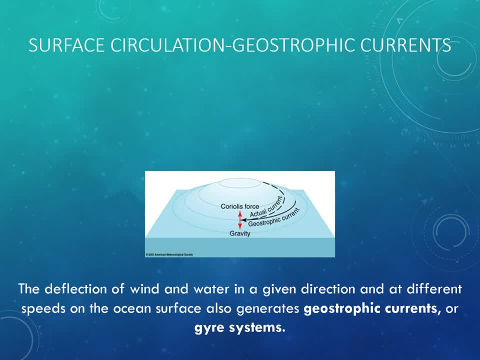 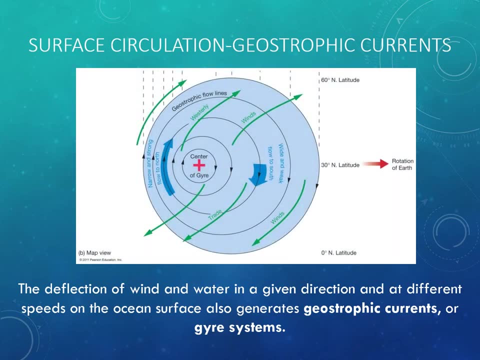 Coriolis Serif Coriolisup force. Coriolisidir positivo Glycine. Coriolis button isn't сегодня opposite direction as gravity and it's going to create the central hill of water that we observe, which, from an aerial view, generates this circular form known as a gyre eastern boundary currents. 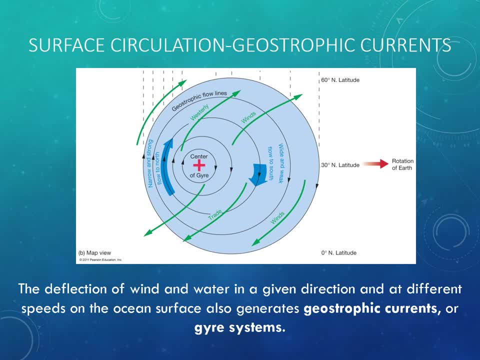 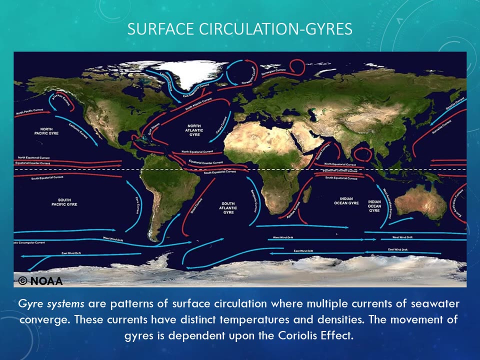 in a gyre move slowly and western boundary currents move quickly. these differences in motion, and gravity again, are what generate that center, the central hill at the center of that. gyre systems are patterns of surface circulation where multiple currents of sea water converge. these currents have distinct temperatures and densities, as shown on this map of the world. 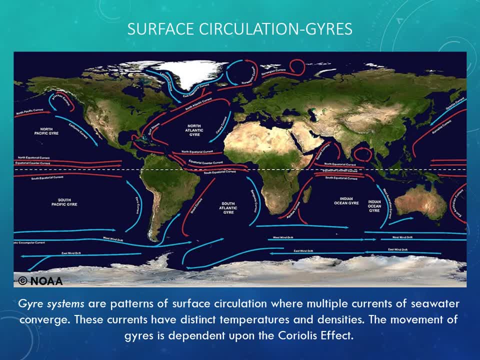 the movement of gyres is dependent upon the coriolis effect, so in the northern hemisphere winds and waters are deflected to the right, and in the southern hemisphere winds and waters are deflected to the left. there are five gyre systems around the world, and they're divided according to. 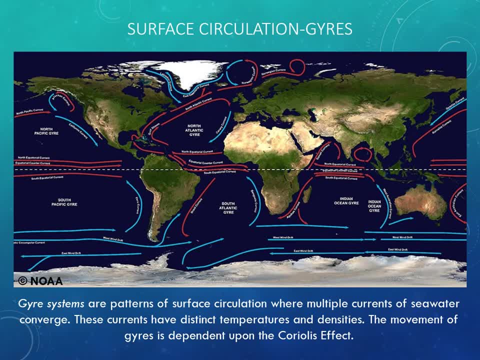 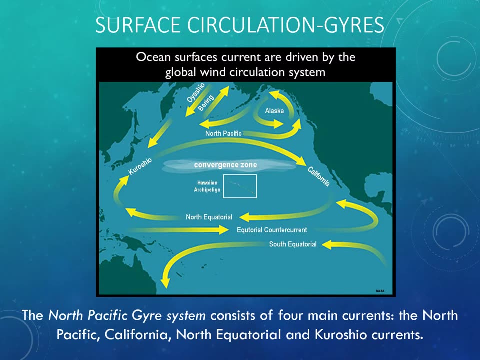 either the continental and continental atmospheres or the pacific and atlantic. so we have the north pacific, the south pacific gyre, the north atlantic south atlantic gyre. we also have the indian ocean gyre. the north pacific gyre system consists of four main currents: the north pacific current, which 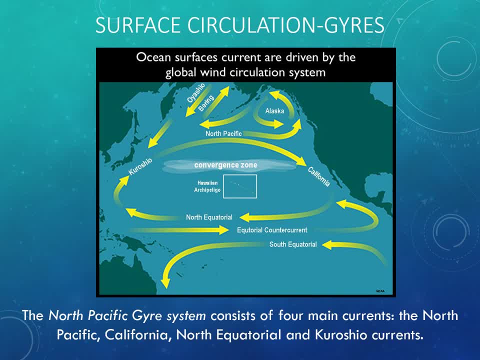 flows in the northernmost latitude around 60, between 30 and 60 degrees. We've got the California current, which flows southward from the North Pacific along our coast, the North Equatorial current which flows westward and the Kuroshio current which flows northward along the Japan coast. North Pacific current is 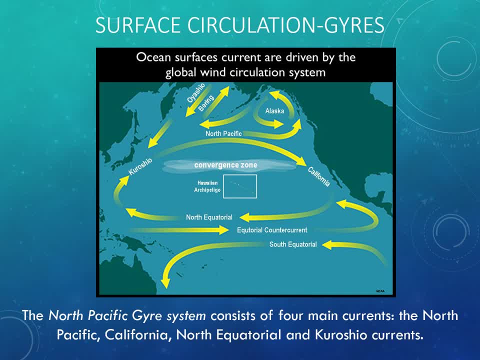 a cold water current. so is the California current, North Equatorial current, because it's flowing along the equator, generally has warmer water And that warm water, as it flows northward, actually moves very quickly Because- remember again, the eastern boundary current, here is the 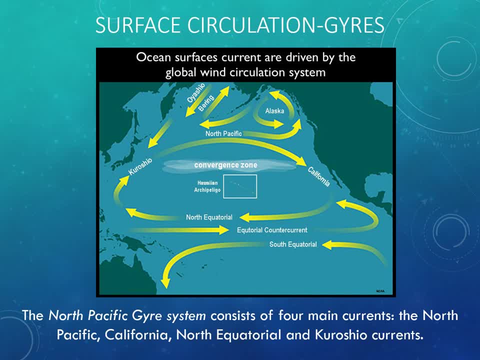 California current flowing much slower than what we have in the west with the Kuroshio current. So these differences in speed have an effect on the temperature variability of each of those oceans along those, each of those sections of the Pacific Ocean, along those coasts. 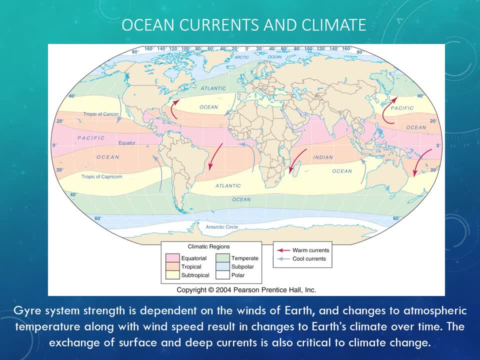 Geosystems strength is dependent on the winds of the Earth. Changes to atmospheric temperature, along with wind speed, result in changes to Earth's climate over time. The exchange of surface and deep currents is also critical to climate change. So on this diagram we have different climatic. 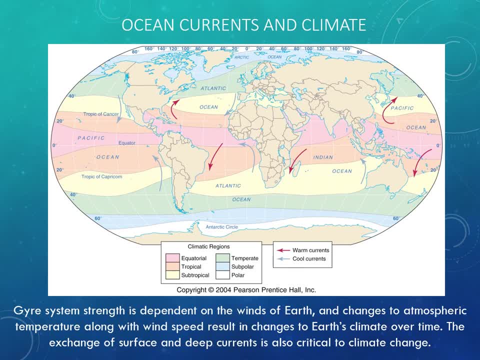 regions of the world's oceans. We've got equatorial, tropical, subtropical, temperate, subpolar and polar. You'll note that along the equator we have equatorial subtropical and tropical climates, So those are generally humid and hot. As we move into the 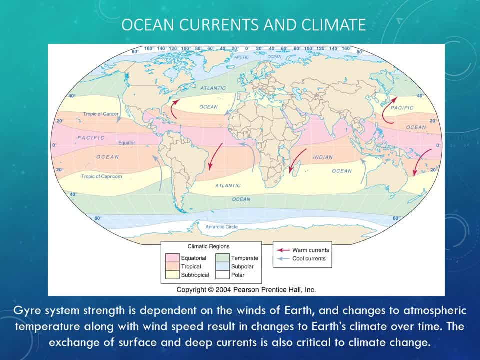 greater latitudes. that temperature will begin to cool off And the air mass will also begin to lose its water. It'll become more dry over time until we approach the poles, where again there's excess moisture that is absorbed, And those air masses are cold and moist And so there's a lot of excess. 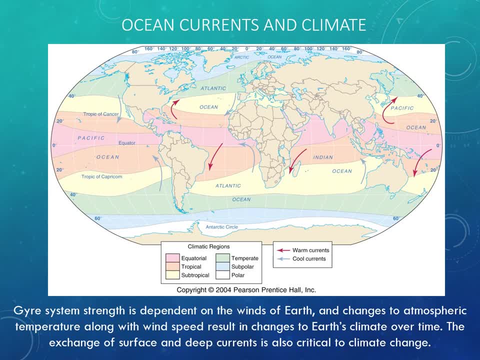 snowfall at the greater latitudes, And so there's a lot of excess snowfall at the greater latitudes over its surface. So changes to these climate latitudes are going to happen as the sea surface temperature increases. That means those bands of, let's say, equatorial tropical climatic regions. 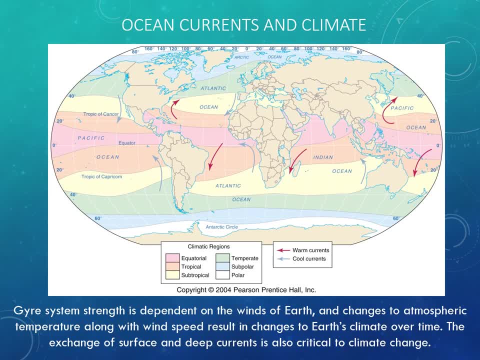 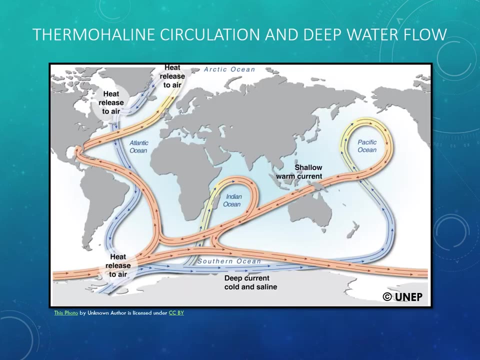 are going to increase. Thus, at higher latitudes, like 20 and 30 degrees, we're actually going to get more humid climate over time than is expected or is normal for where we are in the subtropical desert belt. Now, that's all surface circulation. So gyro systems, what I've been describing to you so far are part of surface. 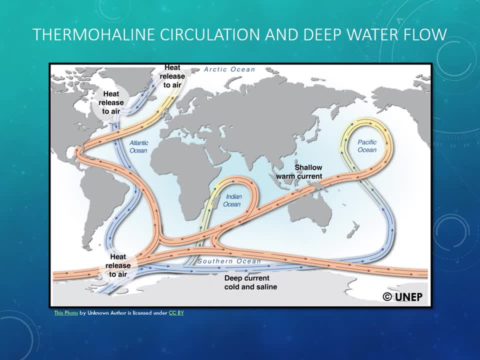 circulation of the world's oceans. Recall what I brought up at the beginning, which is that there's not only surface currents, but there's also deep water currents. Deep currents develop due to differences in solidity and temperature of the water. This generates a phenomenon known as 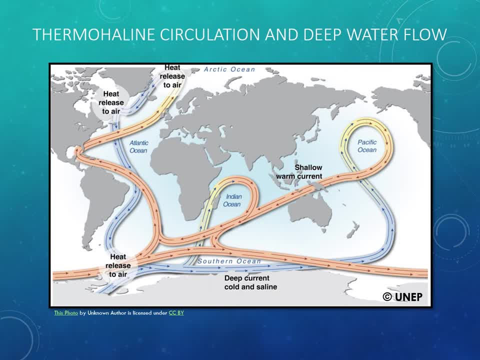 thermohaline circulation- Thermo meaning temperature haline referencing salt. So deep water currents contain excess amounts of salt in their flow. This is because deep water currents originate at the poles. So at the poles, what's happening is that surface ocean water is freezing As it freezes into sea. 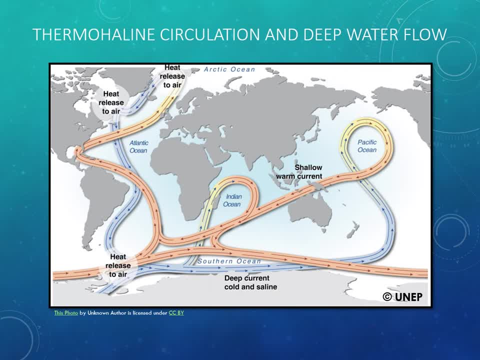 ice, excess salt in the ocean surface begins to sink to the depths. So deep water currents carry those incredibly cold deep saline waters from the poles All the way down towards the equator. So at the ocean basins we have these deep water currents that are flowing and they carry different amounts of. 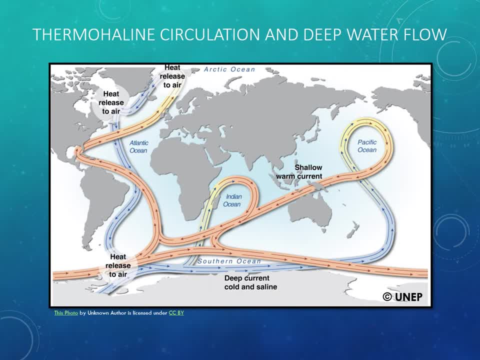 salts, different amounts of other particles, things like dead phytoplankton and dead zooplankton and various other bits and pieces of sediments and other organisms. Those currents are carried in incredible depths in the ocean And again they meet at the equator, where they're extremely cold, So deep water currents are. 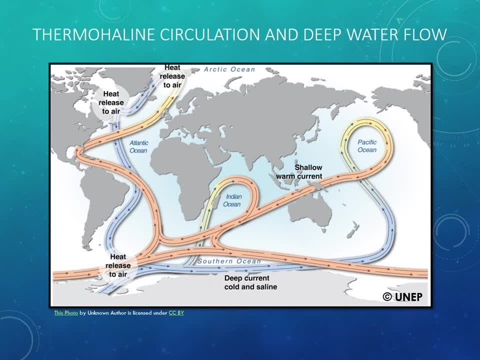 exchanged with surface waters And that's what generates the circulation pattern. So this is the circulation pattern originated around 2 million years ago, when the Atlantic and Pacific Ocean current flow was cut off from each other. Prior to that point, there was an exchange between Atlantic and Pacific Ocean flow. That's no longer happening. 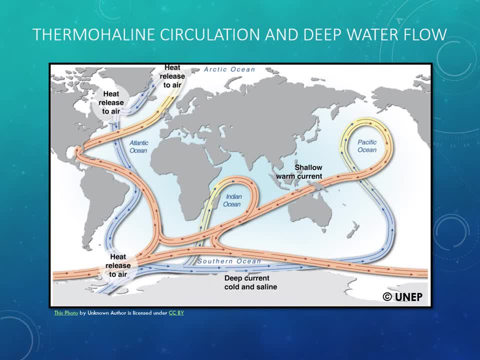 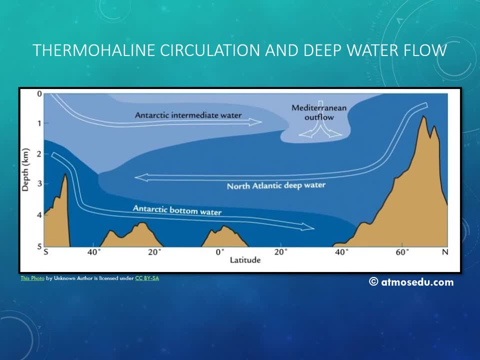 And so what's happened now is this type of thermohaline circulation we have shown on this diagram from the UNEP. There's many types of deep currents or bottom waters, intermediate waters and surface waters in the ocean. This diagram shows the interaction between three types of deep water currents in the Atlantic. 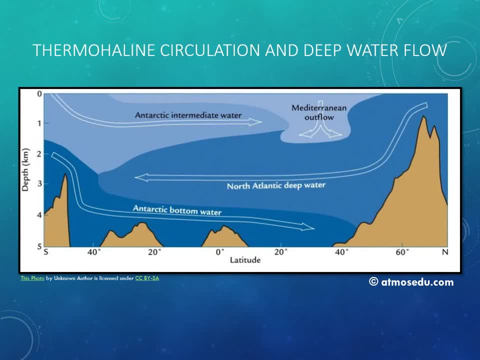 So we've got the Antarctic bottom water current, which again originates from Antarctica from the south, The North Atlantic deepwater, which originates from the North Pole, And then we have the Antarctic intermediate water, which originates again from Antarctica, As well as What's been called today앤ναί ק Lena'a. 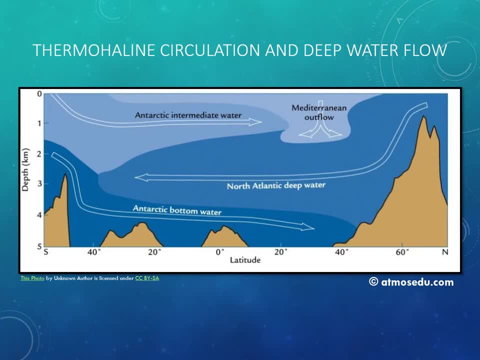 well as surface waters from the Mediterranean. so all of these waters mix at the equator. and again, the deep waters flow from the poles to the middle of the earth surface, and again this is due to patterns of Earth's rotation and patterns of oceanic and atmospheric circulation. each water mass is suspended. 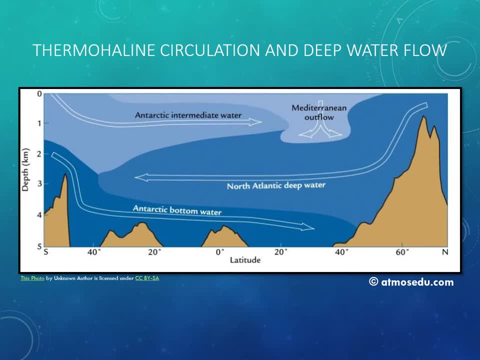 above the other. in order of density, the Antarctic bottom water, referenced as a AABW, is colder and saltier than the North Atlantic deepwater- NADW, which, in turn, is colder and saltier than the Antarctic intermediate water, AIW. so as these water masses converge with each other, there's distinct differences in. 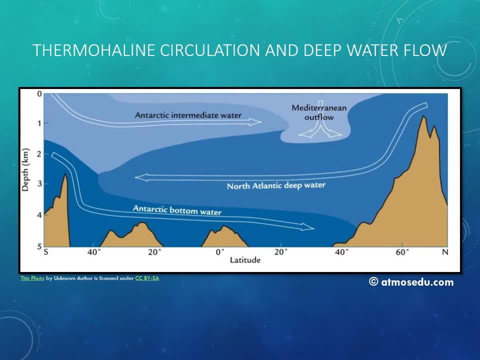 their densities, the Mediterranean outflow that's here in warm surface waters they mix with the deep waters at the equator and so that shows again this thermohaline circulation, how critical it is for the mixing, overturning of these deep waters with the surface water, because this process 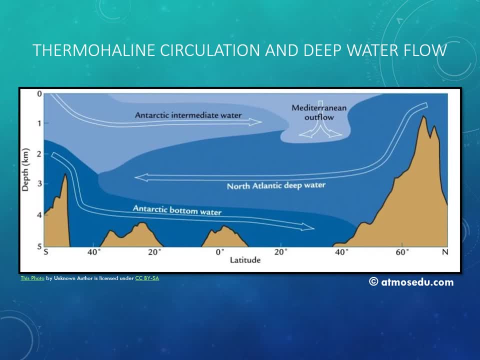 of overturn allows for these very rich sediments and salts to rise to the surface. it allows for particular phytoplankton and other organisms to thrive in different environments, different times of the year, and so, without thermohaline circulation, oceanic ecosystems as we know it would. 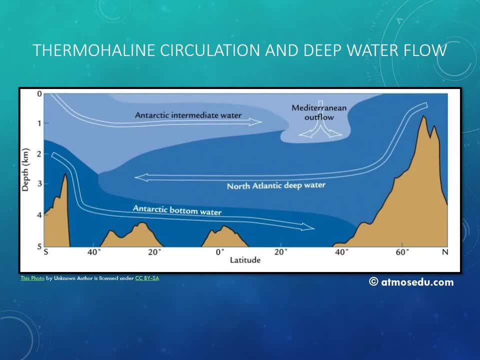 collapse, and in fact this is what happened during the Permian mass extinction event. it's theorized that this phenomenon, similar phenomenon, had happened where this exchange of deep water and surface water stopped. mixing of the ocean stopped, and so when the ocean does not mix any more, then again ecosystems slowly begin to collapse from the bottom. 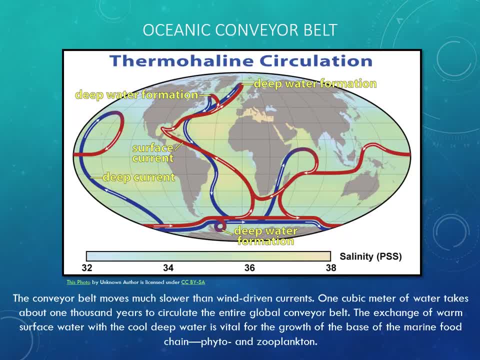 up in terms of the food chain. so the conveyor belt moves much slower than wind-driven. currents. depending on flow, temperature variability with seasonality, depending on, again, sea surface temperature, and mixing all of these phenomena control this process of thermohaline circulation. what's interesting to note is that when we get 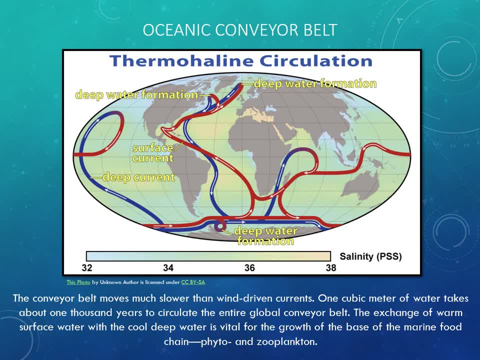 into the deeper water of the ocean. one cubic meter of water takes about a thousand years to circulate in the global conveyor belt system. now, this information is also important in understanding of the outflow of oceanic pollution, which I'll mention at the end of the lecture. 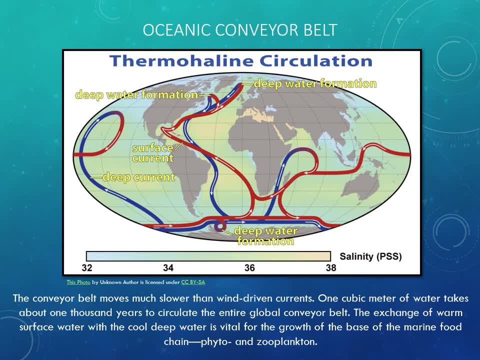 so this exchange again is vital for the growth of the base of the marine food chain, that's phytoenzyme plankton. for more information about marine life in the ocean, feel free to go ahead and check out my oceanography lecture series, which is posted on YouTube under the oceanography playlist. 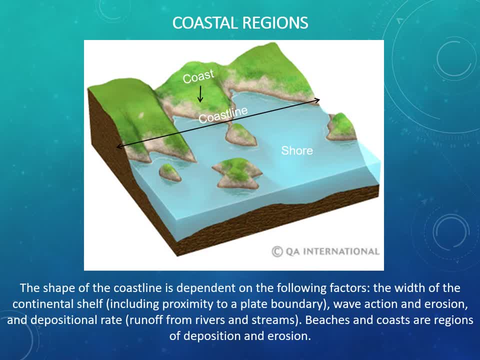 so, with all of this flow of surface currents, with wind and wave patterns that we've learned about in the previous lecture, and with this understanding of how currents work, water currents are an excellent way for which the coastline to be shaped. so what exactly is a coastline or shoreline? 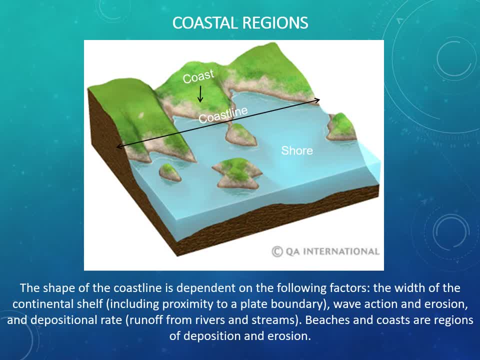 because those terms are interchangeable. well, when we talk about coastlines, we're talking about three parts to the beach, three parts to the essentially coastline area. so we have the coast, which is the land surface, we have the shore, which is the sea, the ocean itself, the shallow sea, and 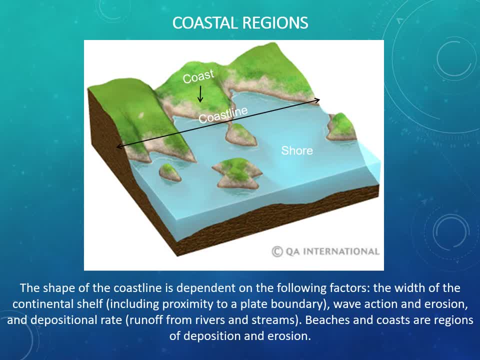 we have the coastline or shoreline, which is the boundary between those two. so coasts are shaped by the wind and water primarily, so wave action will sculpt out the coast over time. however, coastal shape is also determined based on the continental shelf shape. so some coastlines have wide continental shelves. 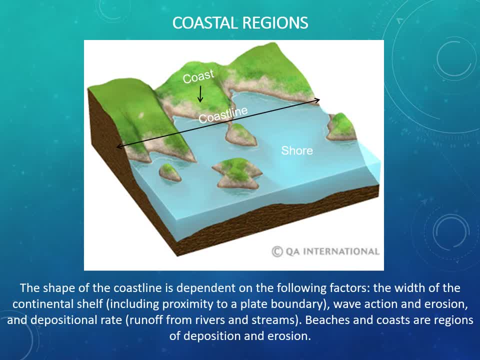 and some coastlines have narrow continental shelves and this has an effect on the different features that we can observe on the coast itself. so the coast is the land surface. again, the shore is the water and the coastline, or shoreline is the boundary between the two coastlines. 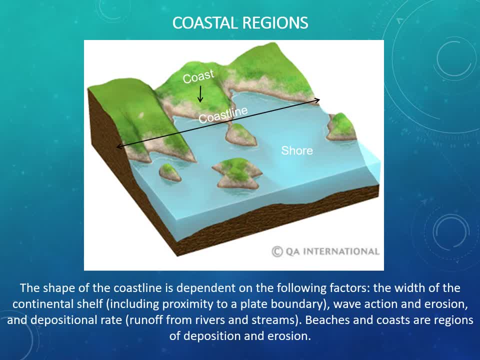 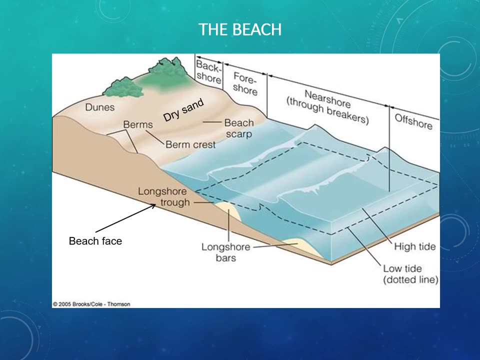 themselves are areas of deposition, in which sediment such as sand becomes deposited in a region that we call a beach, and this sediment is subject to erosion not only due to wind and water, but also due to wave action on a daily basis. this diagram of a beach shows: 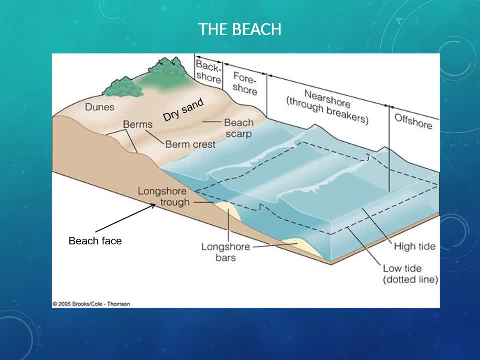 many terms. let's start with the shore or shallow sea. on the right, there's four portions to the shore: offshore, where the fully developed sea ends. near shore, where breakers form. near shore is also referred to as the surf zone. foreshore, where the beach sand begins. features like berms- think of a berm is almost like a line of sand. or 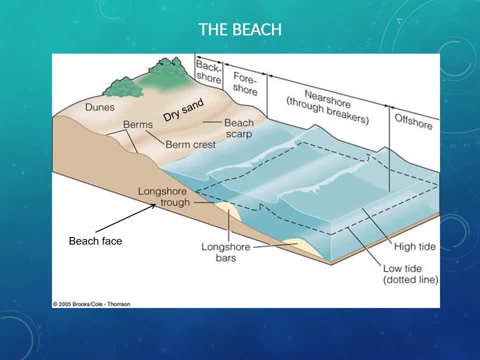 sediment okay, and scarps can form here and the backshore. this is where the water line ends and sand dunes can begin to accumulate and form in this part of the beach. this diagram also shows the level of high and low tide, as well as longshore bars. bars are like berms. there are lines. 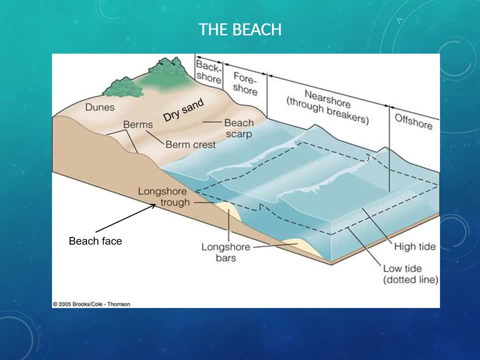 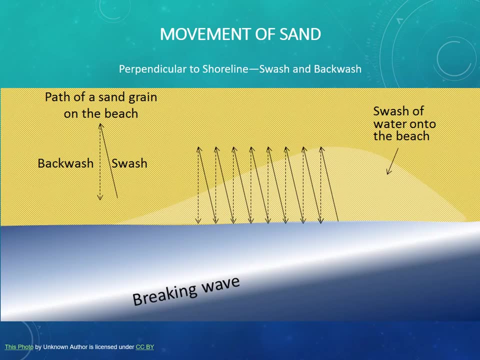 of sediment that accumulate, but in this instance they accumulate due to longshore current. as waves crest and hit shore, they bring sediments such as shells, sand and mud along with them. the movement of sand that's perpendicular to the shoreline is called swash and backwash. 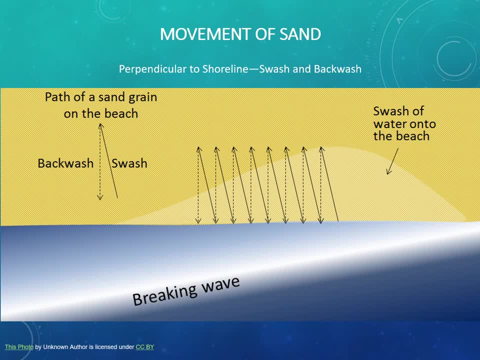 this illustration shows the motion of swash, which is away from the breaking waves and onto land, and backwash, which is moving back towards the breaking waves and out to sea. so there's this constant perpendicular flow of sand. again, that's referred to as swash and backwash. this slide shows swash. 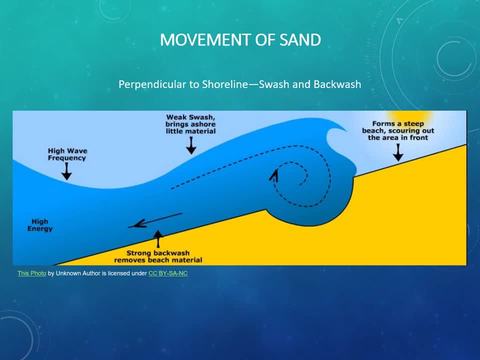 and backwash. another illustration, this time along a sloped beach face. the greater the energy of the wave, the more that the beach face will be eroded by a strong backwash flow. this slide has a photograph of swash and backwash on a flat beach. the energy from the waves dissipates. 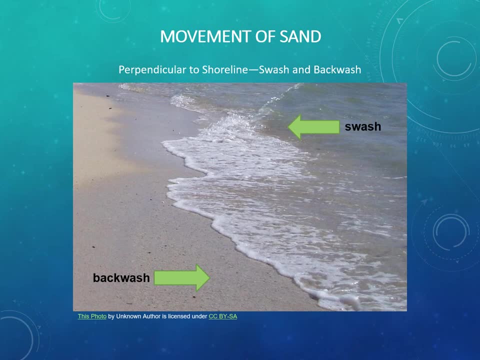 totally as it approaches land, creating very little erosion, unlike the previous slide. so we call that waves themselves, whether they're ocean waves or sound waves. that's energy displacement. okay, so as waves approach land, what's happening is that frictional force is going to cause the wave. 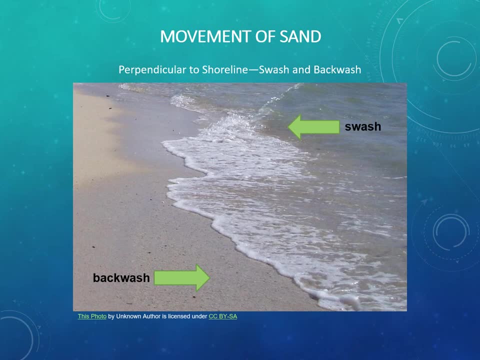 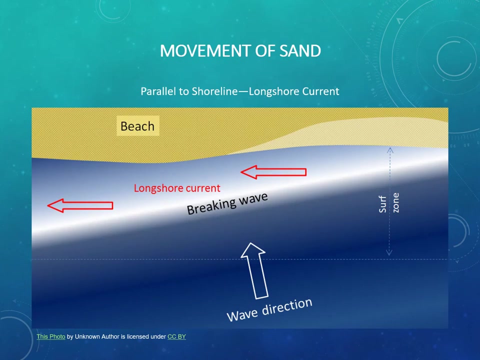 energy to stop or slow down And that's what's going to cause the shape of those waveforms to change. And swash and backwash is just one example of that exchange of energy between the land surface and the ocean. This slide shows the other change of energy that happens as the waves move inland and that's known as longshore current. 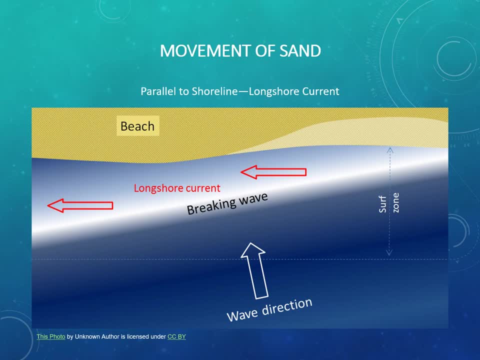 Now, one of the dangers of longshore current is a phenomenon known as rip current. So rip tide or rip current happens as longshore current moves parallel to the beach. Longshore current itself is a flow of water, So it's the flow of seawater that's moving parallel to the beach. 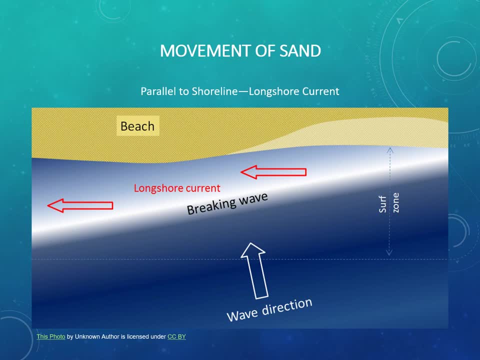 Longshore drift is what happens when longshore current, as it moves, deposits sediment along the coastline. So note that longshore current is parallel to the beach face And, as the waves break and as they move towards the land, that swash and backwash pattern that we observed in previous slides, that pattern is perpendicular. 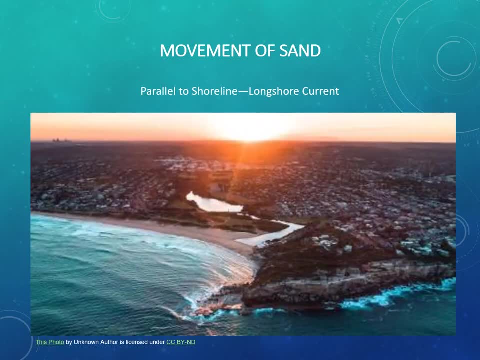 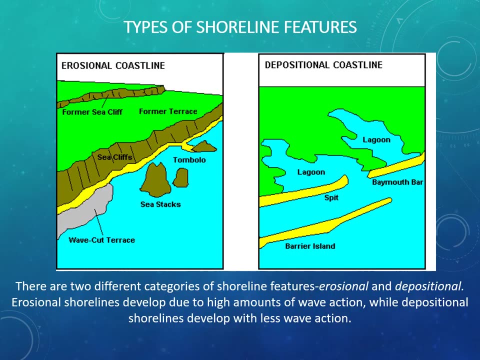 In the surf zone. This slide has a photo of longshore current that's moving parallel to the beach. So as waves break in the surf zone and as they hit land surface again, and because of the differences in the shape of the continental shelf and slope, you get differences in the type of coastline that we can observe. 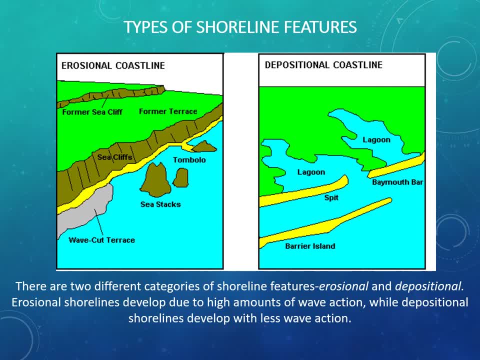 There's two different categories of shoreline features that exist, And these are classes, Either erosional or depositional. Erosional shorelines develop due to high amounts of wave action, while depositional shorelines develop with less wave action. These images depict different features in each type of shoreline. 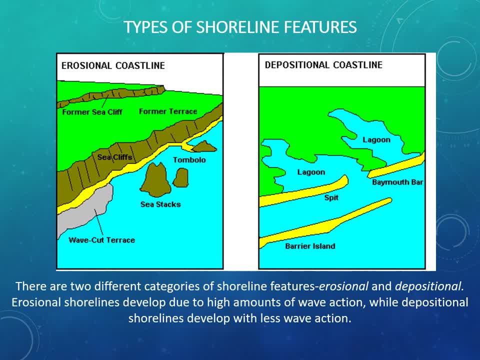 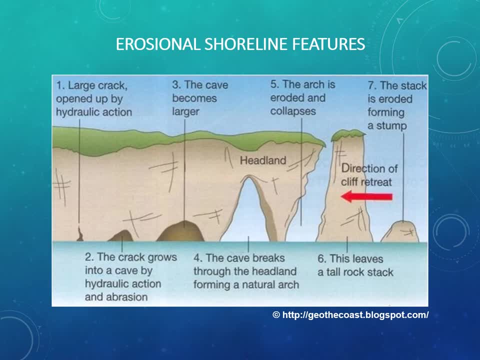 Let's discuss erosional features first. Erosional shorelines tend to have narrow beaches. They have narrow continental shelves that are steeply sloped. Erosional shorelines have large cliffs that are eroded by waves in the surface. The coastline is a here and there zone. 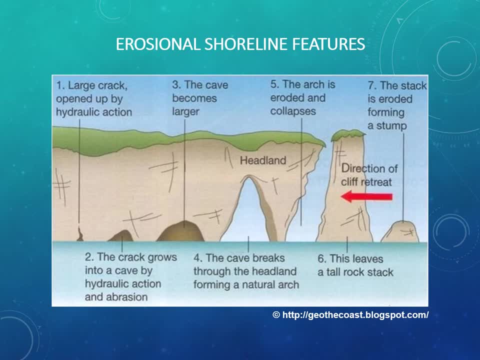 So we've got large cliff, narrow beach, and then there's the ocean, And that's what most of our coastlines are like. in Southern California, Most of the time we have erosional coastlines or shorelines here. So as the wind and water hit the surface of the rocks and the cliffs, a process known as abrasion will occur. 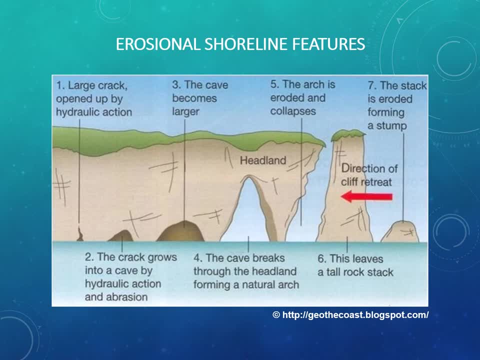 Abrasion is when rocks collide with one another and they break down into smaller pieces. So as the waves break and hit the slope of the land surface, we'll have a lot of erosion. So as the waves break and hit the slope of the land surface, we'll have a lot of erosion. 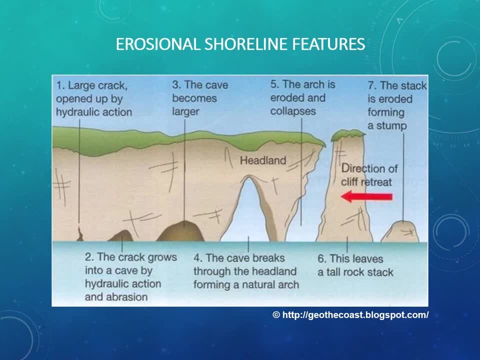 We'll have a lot of erosion. sediment carried in those waves will hit the sediment that's already on land and in this way it'll slowly grind down the land surface and especially this will especially affect softer sediments. so things like buds and silts are more. 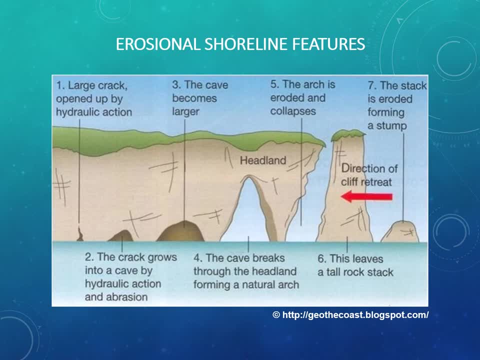 readily affected by this process than, say, you know, coarser grain sands or possibly conglomerate type gravels, right those types of energy, that type of energy is different there. so the energy from waves in the ocean can also break down rock surfaces itself over time, sometimes through salt as well. the salt 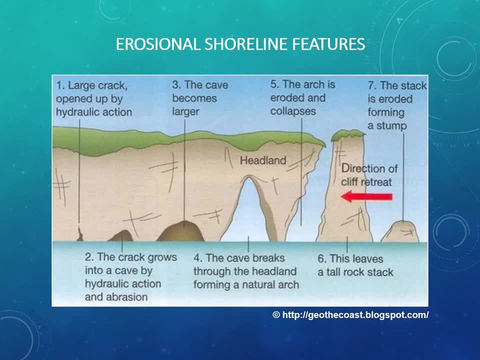 that's present in the ocean can also gradually erode rock, and so that process- where you know, waves are just crashing against the side of a cliff- that's known as hydraulic action. so, taken together with both abrasion and hydraulic action, what happens is is that cracks and crevices and the rocks can begin to form. 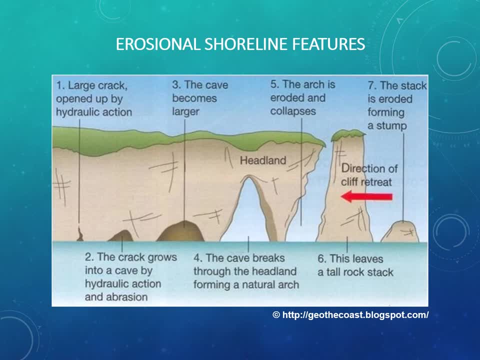 the cliffs and those can eventually grow into caves and then arches and over time, with erosion of the topmost portion of that arch, stacks can form. so this illustration shows how that process of repeated breaking of waves on the cliff can develop each of those features that we find in an erosional shoreline. so 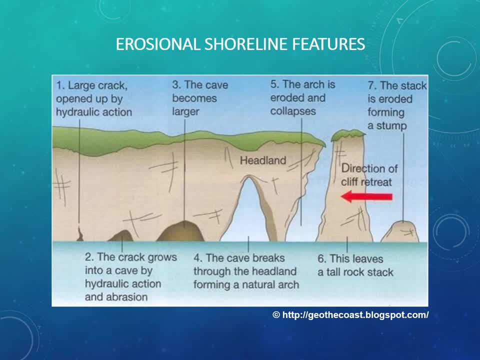 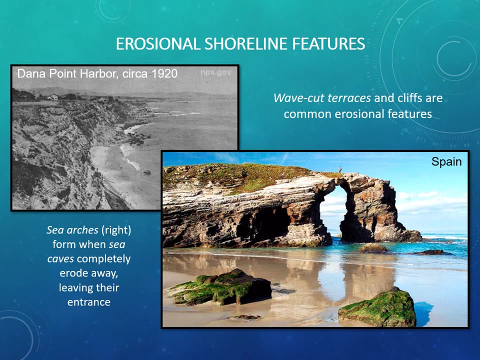 gravity, wind and pressure will cause the topmost portion of that arch to kind of break away and develop into a column, that of rock that we call a stack. this slide shows some of the original features I mentioned on the previous slide and some photos. we've got a beach. we've got data point harbor from 1920. so 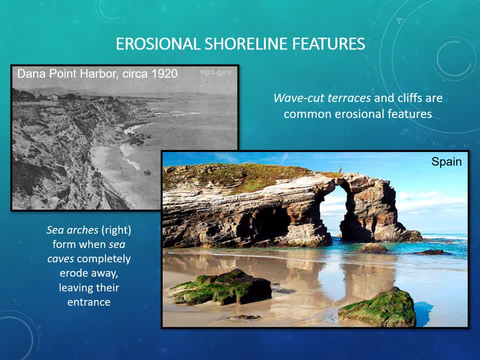 from a hundred years ago. this is what data point look like, and we also have a photo, more modern photo, of Spain with some sea caves and an arch. so the data point harbor image shows some cliffs. they're very narrow beach. we've got what we call a terrace, which is another name for a sea cliff here, and there are some. 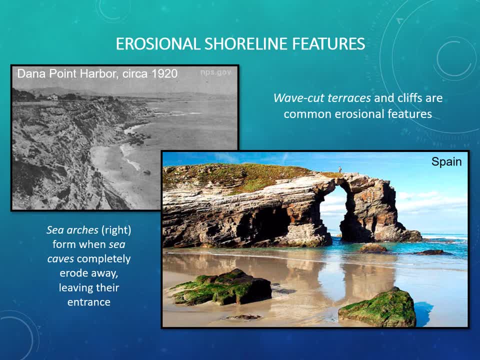 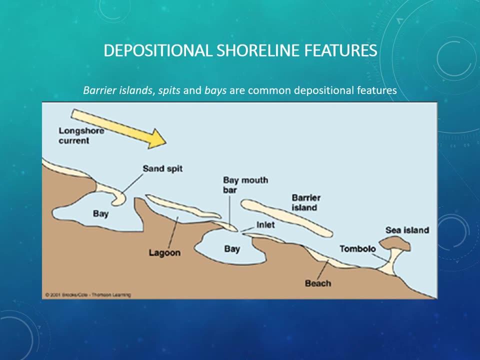 features here, like tide poles and things that still exist, but, as you'll see in later slides, we have modified our beach so it's more depositional than erosional depositional shorelines. they tend to have wider beaches that are more tidally dominated, and this happens because these beaches form on wider continental shelves and these shelves are more gently sloped. 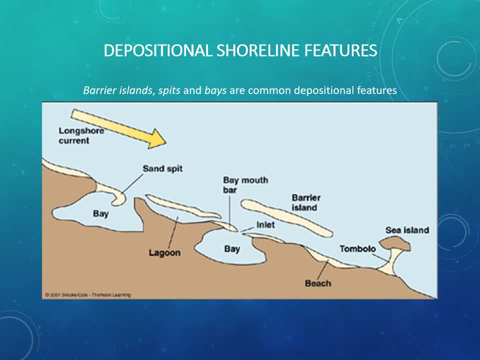 this allows sediments to gradually build the coast over time, especially as rivers empty out into the ocean. depositional shorelines are defined by these features. here they're shown on this image. we've got some lagoons, embayments and barra islands on this illustration, along with longshore current, so 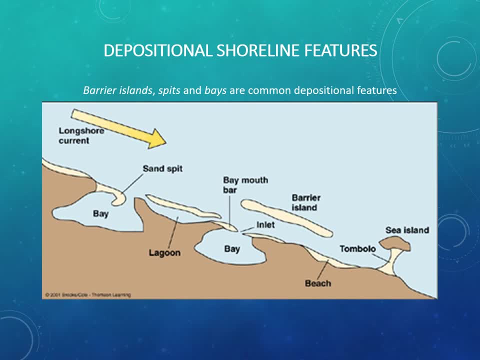 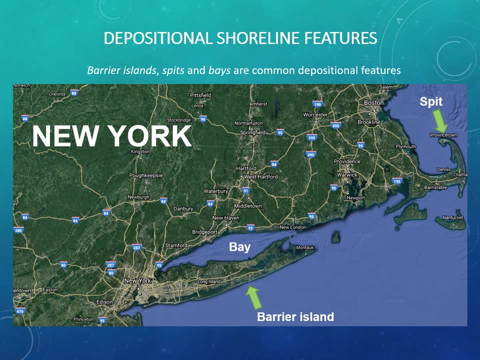 longshore drift and longshore currents are what help to build up these depositional shorelines over time. now we don't really have a whole lot of depositional features here. we do have a few that are left over from the 1800s, that are remnants of what used to be here, so hundreds of years ago our coast was a. 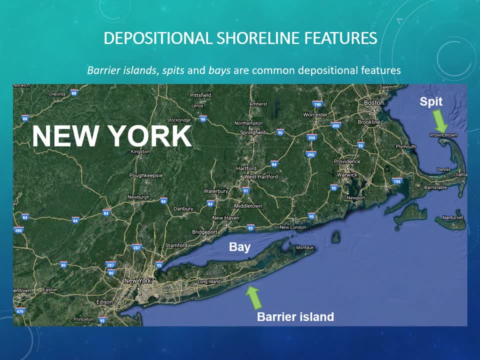 natural depositional coast, but we've since altered it and i'll talk about that in a little bit. so instead let's go to the east coast. so on the east coast, united states, there tends to be a lot more depositional features, depositional shorelines. so this slide shows the coastline of 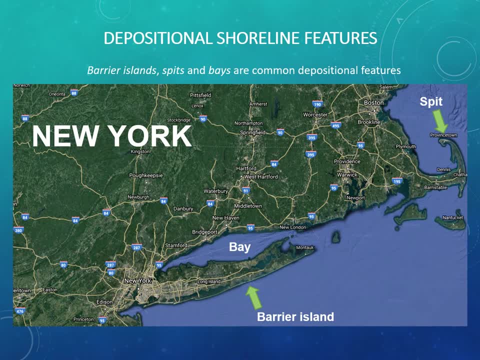 the state of new york. long island is a barrier island- barrier islands developed due to excess sediment, usually by longshore drift. this island cuts off the flow of the atlantic ocean and that's what causes water to kind of refract or bend around the barrier island and lose energy as 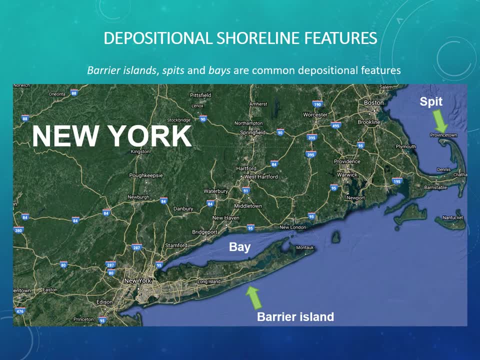 it crests on shore. this excess water will then collect in a region that's known as a bay. so that bay, that abatement there is some of the, is still connected to the atlantic, but it's again behind that barrier island and again because there's less direct contact between the ocean surface and the 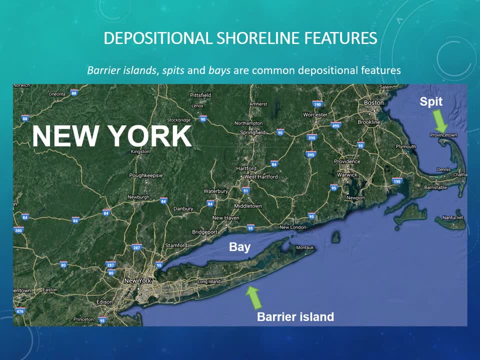 land surface. it's a little bit more tidally controlled. there's a lot more deposition of sediment in this area and because of that wetland ecosystems will form in this way. spits are also areas of deposition of sediment. they form a hook-like shape and again, that's due to refraction. 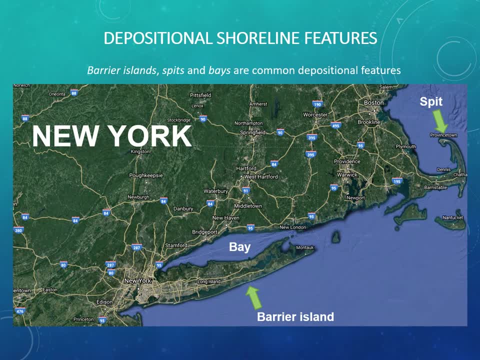 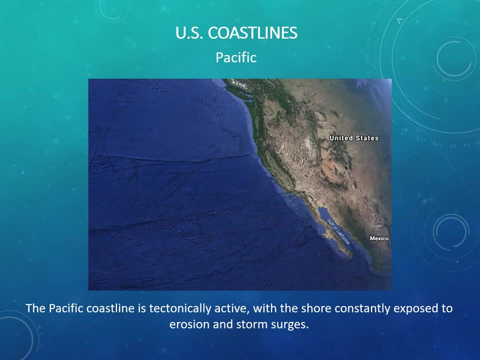 of wave energy as the waves approach and bend around that land surface. most shorelines have a combination of depositional, original features, such as the longshore drift and the longshore drift, and our coastline is no exception. however, one type, whether it's original or depositional, tends 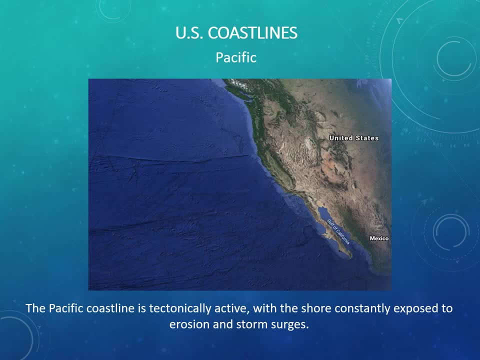 to be more predominant than the other, based on, again, the shape of the continental shelf, wave, energy and also elevation, land surface above or below sea level. so whatever sea level rises, this also has an effect on the shape of the coastline. the next few slides show the coastlines of united 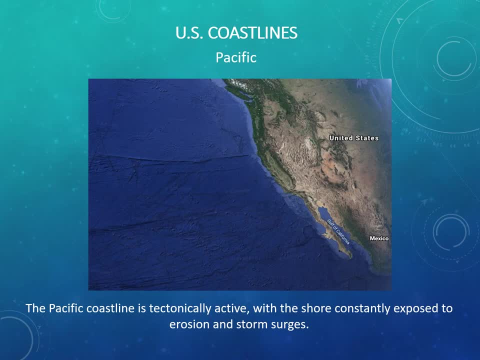 states and whether they're primarily erosional or depositional in the coastal features, starting with the coastline which is our coastline, included. it's tectonically active, so what this means is is that we're not only situated on this plate boundary here. this transform boundary with the san andreas fault. 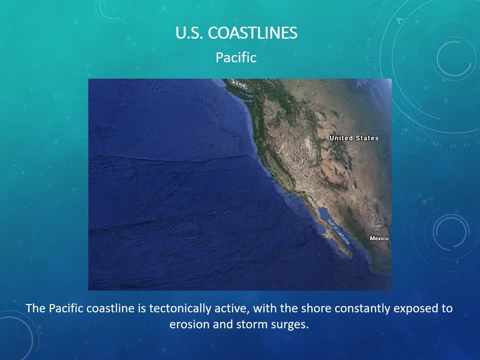 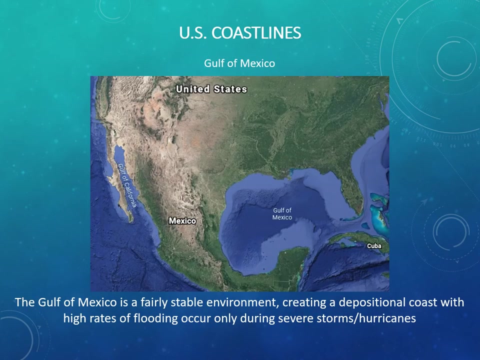 but the shore is constantly going to be exposed to erosion and storm surges, and note how narrow the continental shelf is here. so again, a lot of our beaches and features are erosional features here because of all these processes. the gulf of mexico, on the other hand, is a little bit different. note how much wider the continental shelf is here. 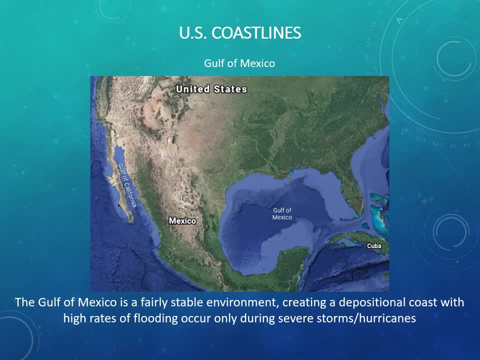 in addition, because of the lack of flow from the atlantic into this region, the gulf of mexico is definitely more tidally dominated, so there's a lot more swamps and, in this case, bayous and other coastal features that we find associated with depositional environments here. 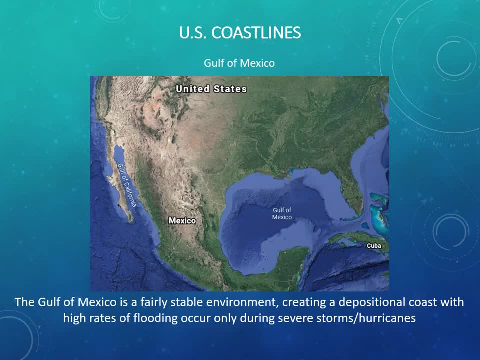 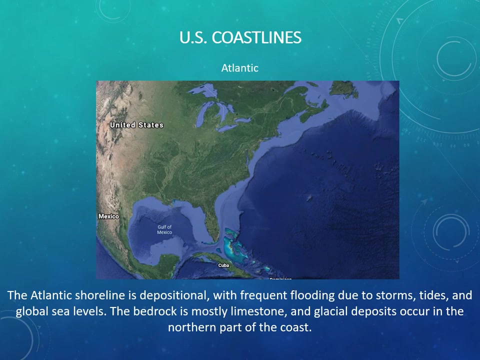 now. severe rates of flooding do occur, typically during hurricane season, during severe storms and hurricanes, but again, for the most part these beaches are depositional in nature. finally, once more we have our atlantic seaboard, so this is the east coast of the us. we've got deposition of sediment here. note again how much wider the continental shelf is here. 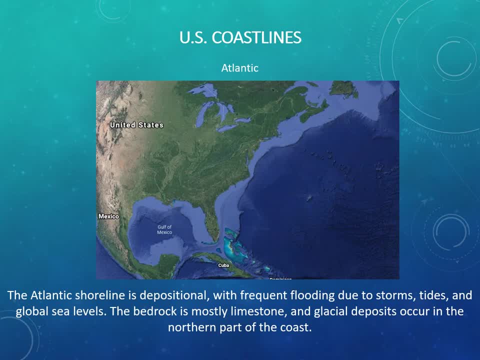 especially by the florida panhandle area parts of the south. you'll note that there's again excess deposition of sediment here. excess swamps and those types of wetland environments can easily form here. so while nature does most of the work in shaping the coast, humans have altered the landscape. 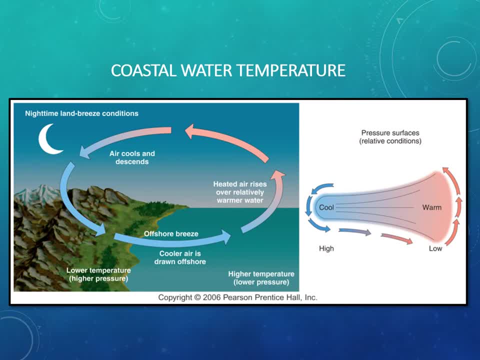 drastically over the past several hundred years, and this is primarily due to the industrial evolution. so, starting in the 1800s, when we started to manufacture things more, cities began to develop and take over various natural environments. people began to inhabit coastal regions more as well. so while nature does most of the work in shaping the coast, humans have altered the landscape drastically. 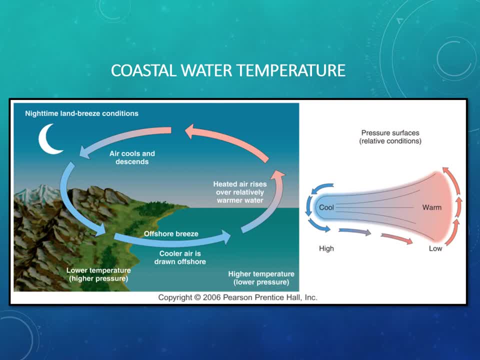 over the past several hundred years, and so people the reason why we inhabit coastal regions and people have been doing this. indigenous people have been living along the coast as well for thousands and thousands of years prior to the industrial revolution, but people have been inhabiting coastal regions primarily due to the mild climate, and the mild climate is, in part, due 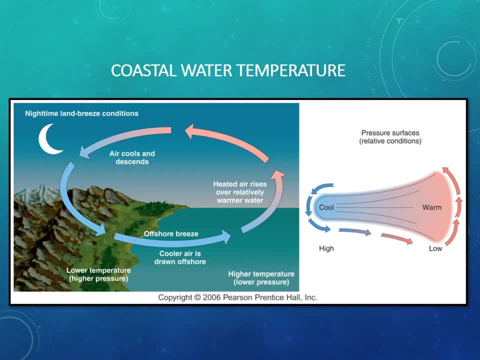 to this process, as shown on this slide, which has to do with temperature regulation. so what's interesting about- well, what's known about- the ocean is that the ocean is a heat sink, right. so the ocean will absorb excess amounts of heat that are accumulated in the atmosphere during the day. 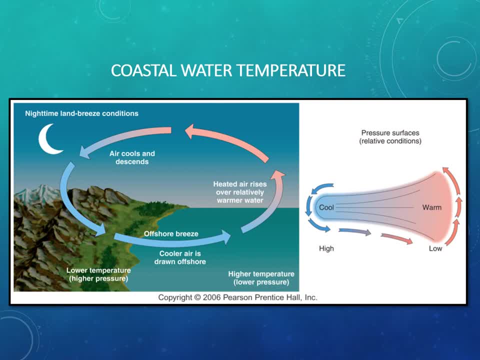 and from this process, the air that flows across the surface of the land- if it's closer to the ocean- is much cooler, and so, because of this cooler air, there's a lot more mild climactic change in temperature here along the coast than what we have further inland. so for people that 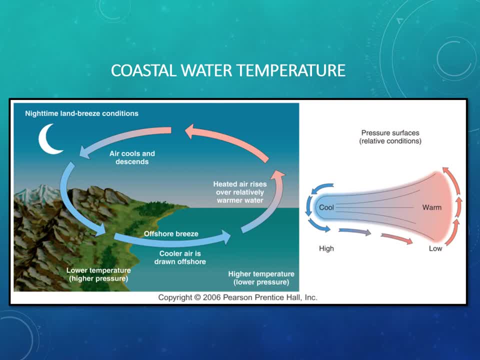 live further inland right, weather tends to be a lot more extreme, so during the day, for example, temperature can skyrocket to over 100 degrees in the summertime, and then at night it can go down to maybe like the 40s or 50s, and these extremes in temperature on a daily basis are much more. 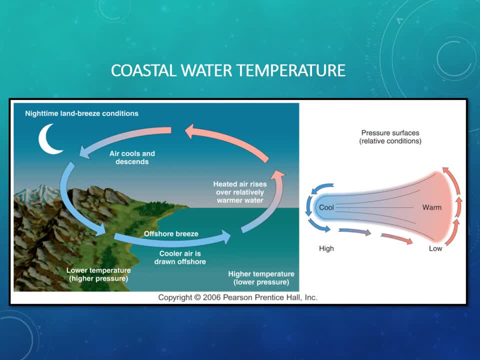 noticeable inland than they are along the coast, and so that's part of the main reason why so many people live along coast globally- not just here in california, but everywhere. so it's a mild climate. it's also an abundance of food and natural resources, like oil and natural gas, which are easily 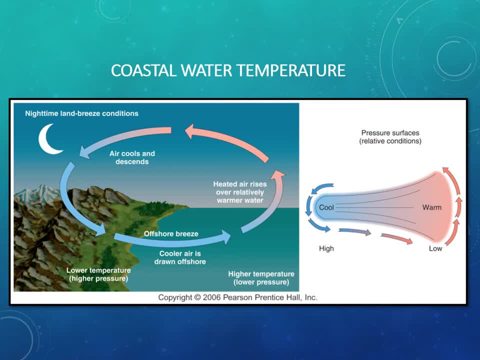 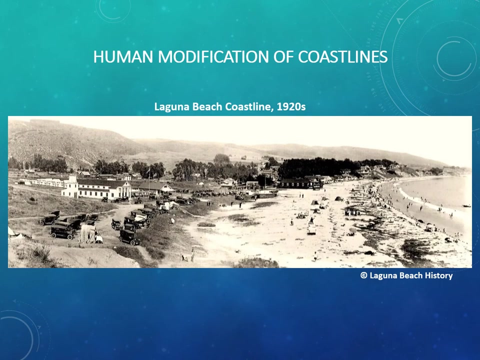 exposed, and also a lot of these things can be extracted from offshore and onshore coastal environments. so coasts have been modified again, since the industrial revolution primarily, and they've been modified to make way for ports, piers and this increasingly dense human population along the coast. on this slide is an image of laguna beach from 1920. 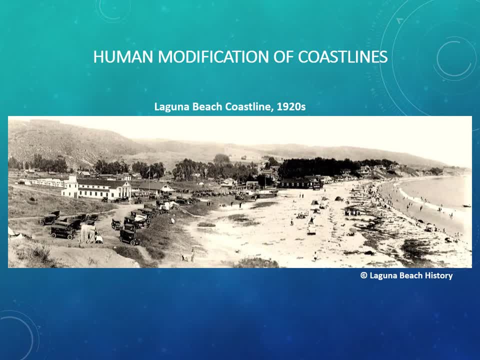 note the position of sea level, the rugged terrain and cliffs, the beach. so here we've got all of these cars parked on the left and we've got people on the right that are heading out towards the beach. notice where the water line is. i notice the housing, the trees, the hills. keep this image in your mind because as i move to the next slide, 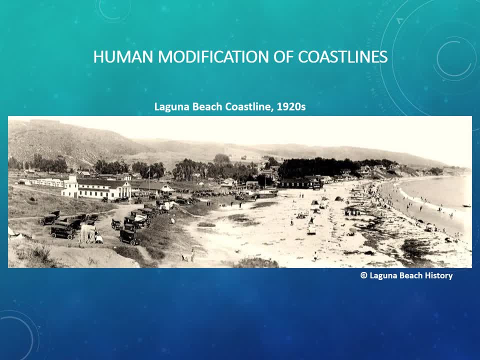 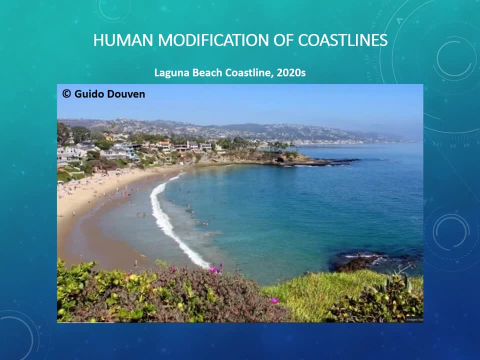 you're going to see just how much change has happened in only a hundred years. so this is what, the same direction. this is what the laguna beach coast like coastline, looks like now. sea level has risen and it will continue to rise in the next hundred years as well. 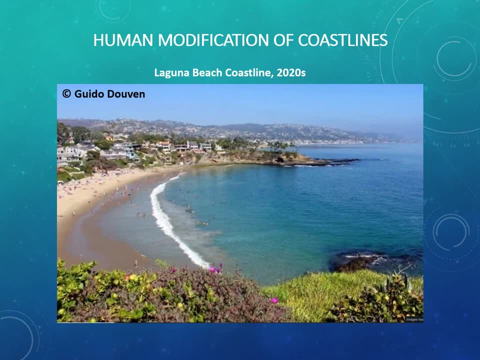 note just how many people now are living along the beach in terms of housing. look how close those houses are to the water line, okay, so notice also that the hills have changed in their shape, right? so the entire coastline has been built on the beach, and i'm going to show you a picture of the coastline. 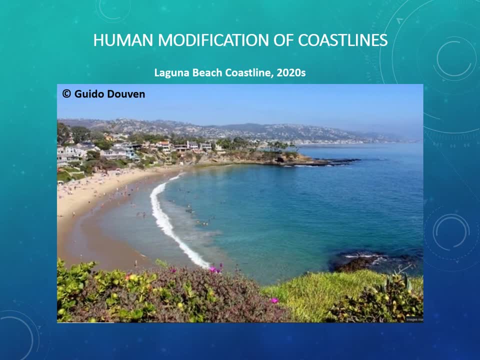 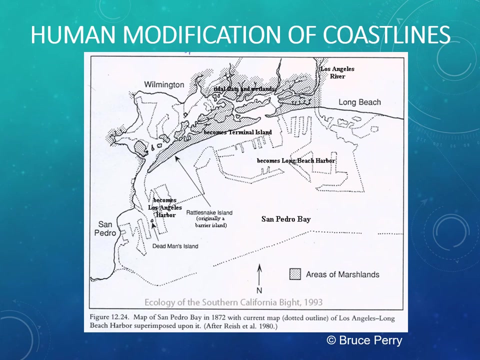 been modified by us. we've changed coastlines again to make way for harbors and ports, like the port of la port of long beach, which are major hubs for economy, but at the same time we've drastically altered our landscape permanently. this slide is an illustration of southern california coastline as it was in 1800s. 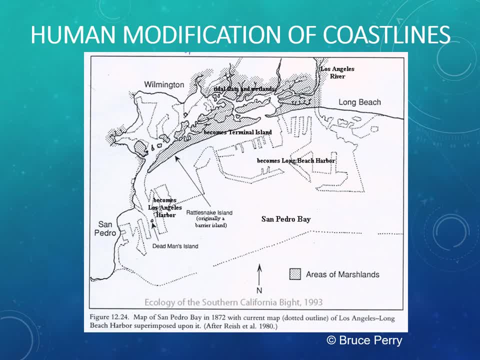 so the dashed lines here, or dotted lines, represent the placement of the ports of la and long beach. sections of san pedro as well are shown here. i noticed that at one time, near 150 years ago, we did have a barrier island here and we had tidally dominated areas. 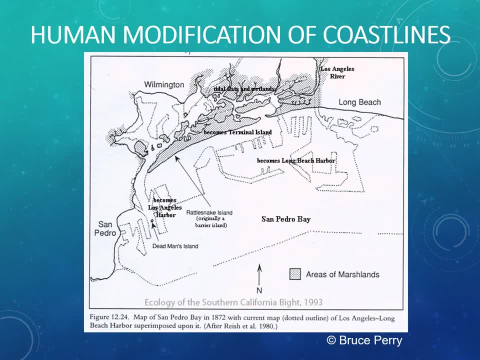 over that span of 150 years, those coastal wetlands that we used to have here from the tidal flats, they've been drained and destroyed, and the rivers that naturally emptied in the pacific have been damaged and had to be removed with a new and new design, and so we've also relaxed that area and 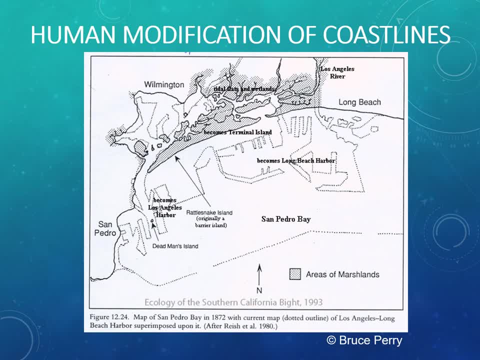 instead we've working to make it a more modern area in terms of making it more down to the diverted and essentially funneled into concrete. so the entire coastal shape, we completely altered and changed it. we destroyed a barrier island here, we took out all the wetlands and this was all to 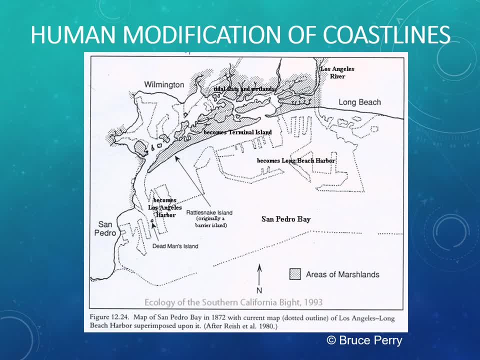 kind of level out and flatten the area so that ports and harbors could have a sense of, i suppose, like normalcy in terms of water level, so that you know as boats can pass through they're not going to say hit like some kind of barrier island or not be able to get in because of excess swampy. 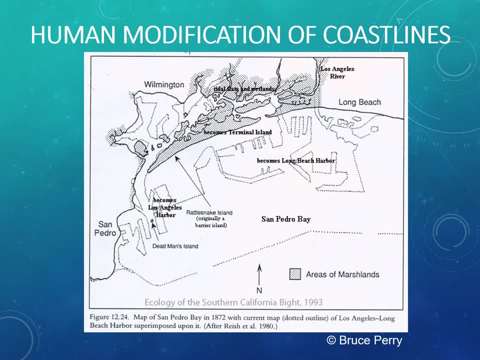 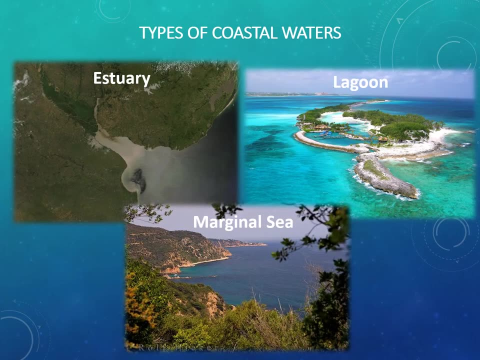 areas right. people could easily traverse the landscape, drop off their goods and go back out to sea once more, and we've been using these ports again for hundreds of years, but at what cost? so coastal environments- natural coastal environments- are categorized into three types. these are estuaries, lagoons and marginal seas. 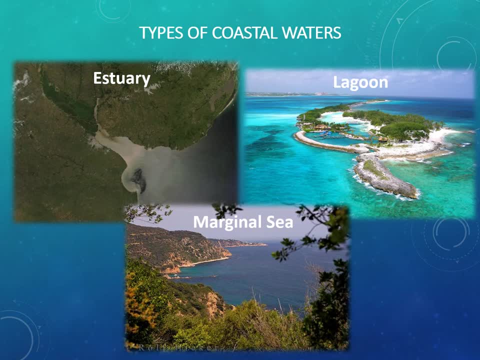 as shown here, as shown on this slide. so we've got an estuary on the left, we have a lagoon on the right and we have a marginal sea in the middle. all of these are tidally dominated environments that connect to the open ocean in some way. 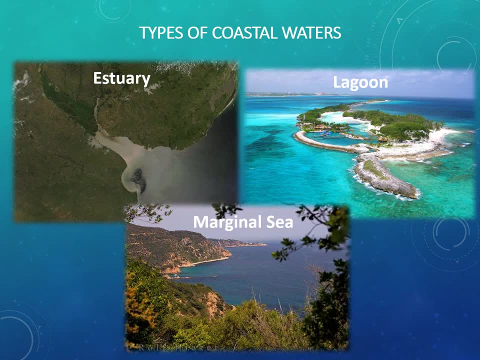 in southern california, we have remnants of estuaries that still exist along our coast, and that's where we're going to focus. our talk for this week is on estuaries and wetlands ecosystems that are derived from them. an estuary is an area of land where river or body of fresh water meets. 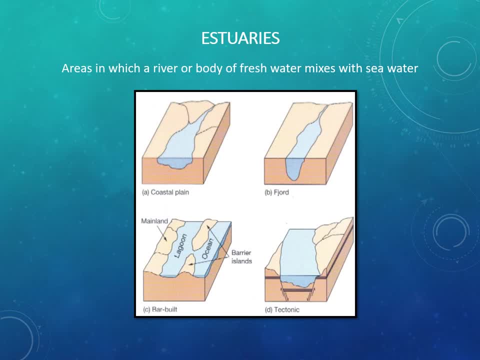 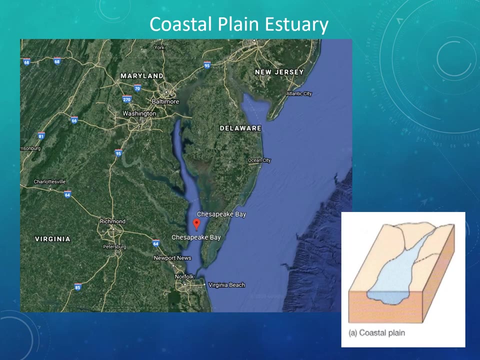 the ocean. there are four types of estuaries as illustrated on this slide: coastal plain, fjord barbilt and tectonic. coastal plain. estuaries like chesapeake bay and maryland form as the river empties out into the ocean. this creates a floodplain environment along the coast and also estuaries can form. wetlands can form in this way. 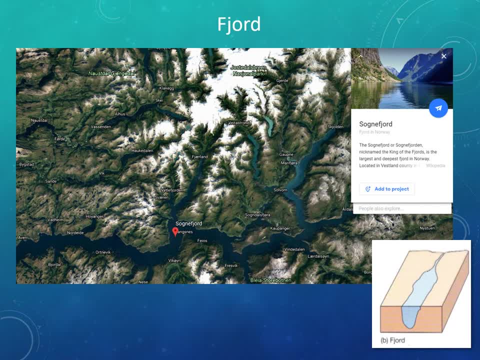 youngman Здобувы. fjords, like the king of the fjords in norway, form as a glacier retreats and that melt water rivers. those rivers will then meet the ocean. so for those of you that are fans of the disney film frozen two, you're probably thinking of that. 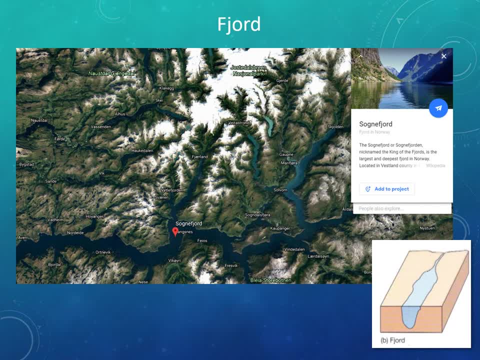 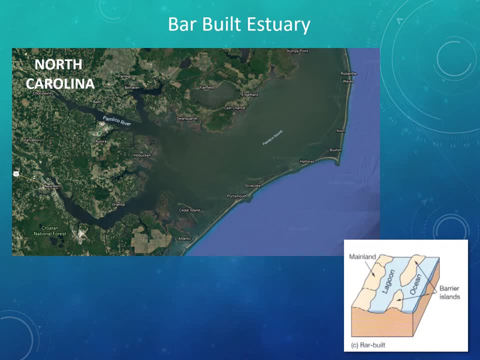 line from the film and that's referencing a fjords in that particular region in norway. expansion to the east: Bar-built estuaries, which are shown here, with Pamlico Sound off the coast of North Carolina they form, as bare islands, block flow from the river into the ocean. 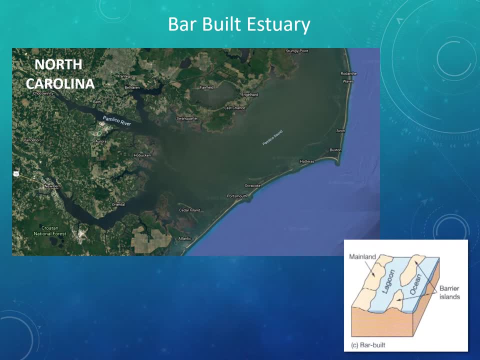 and that creates this embayment or lagoon type of environment. So again, that's a bar-built type estuary, So we've got bare islands or spits, that kind of block that ocean flow and at the same time have enough of a connection to create this lagoon type of environment. 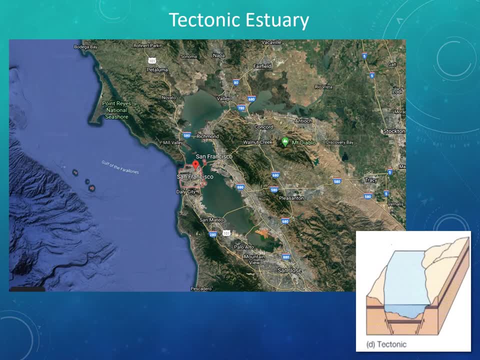 Tectonic estuaries, as shown here with San Francisco Bay Area, develop along fault zones or escarpments. Here the Sacramento River is offset by sections of the San Andreas Fault as it empties into the San Francisco Bay. Most of the remaining estuaries that we have in Southern California are tectonic estuaries. 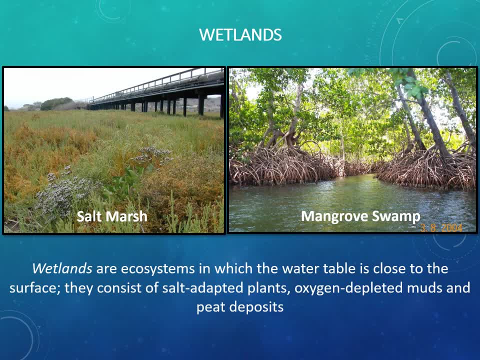 Estuaries can create wetlands. Wetlands, as I mentioned to you before, are ecosystems in which the water table is close to the surface. Most wetlands consist of salt-adapted plants, So in other words, they are adapted to an environment where there's changes in salinity. 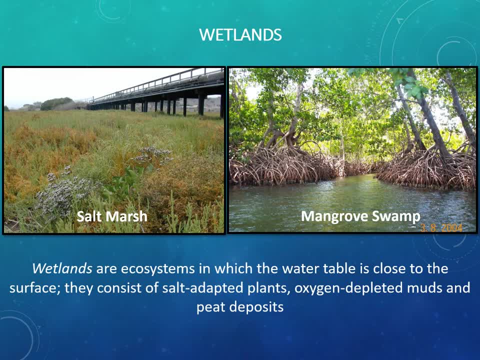 changes in pH because of changes to tide, to tidal level, And they also consist of oxygen-depleted muds and peat deposits. In these oxygen-depleted muds there are various forms of bacteria that can actually consume and destroy various types of marine pollutants that get into sediments. 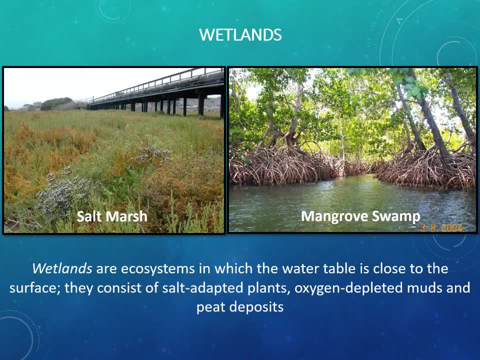 In addition to enriching and recycling muds and plants that are already present in salt marsh environments. This process is known as eutrophication, And it's critical for maintaining the health of the coastal environment. So there's these two categories of wetlands. 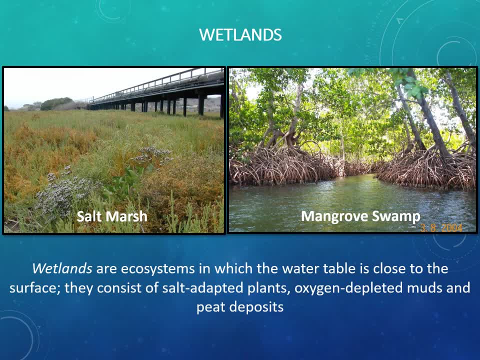 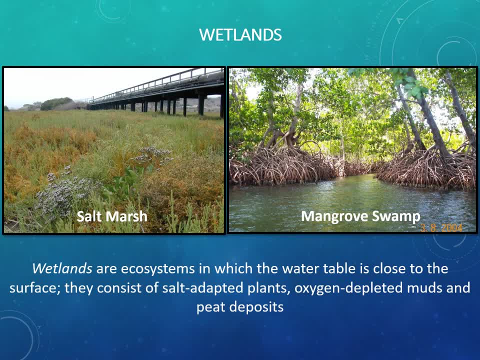 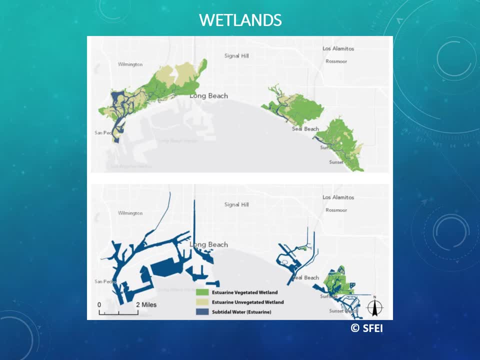 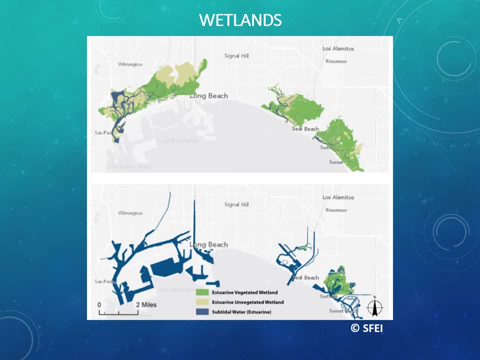 as well as various harbors for boats, including sections of Newport Beach and other coastal environments here, like Naples and things like that. So these images are before and after Southern California's wetlands, with the top image a representation of our coast around 150 years ago. 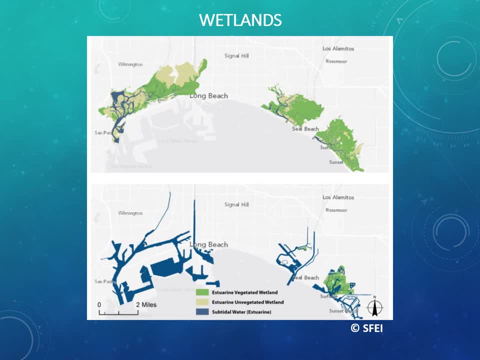 So in green and yellow we have all of our estuaries there, And blue are the rivers that emptied out into the ocean. So parts of the Anaheim River are diverted here with Seal Beach, Parts of the LA River are diverted in Long Beach and San Pedro, And so those rivers have now since been kind of dammed up by concrete And those estuaries, as you can see in the bottom image, are totally drained and destroyed. 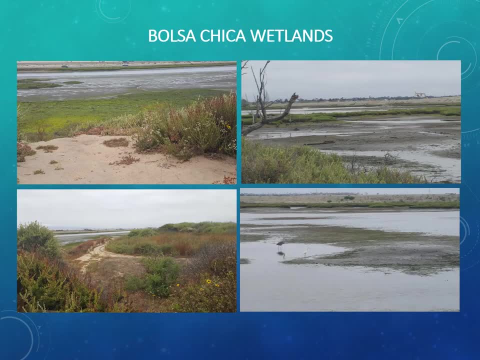 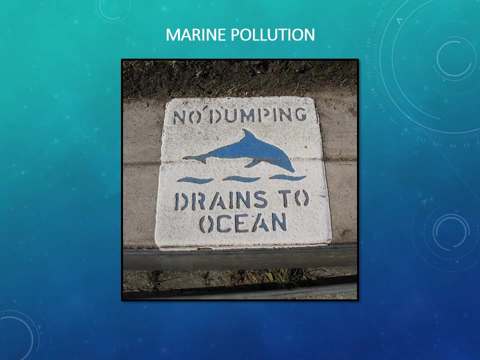 So here are some images of the Bolsa Chica wetlands in Huntington Beach, California. Its over 100 acre reach has now been reduced to only a few acres at best, with nearby property and roads encroaching on the area. As coastal populations increase, we have more of an impact on the oceans. One of the direct effects of this is marine pollution. 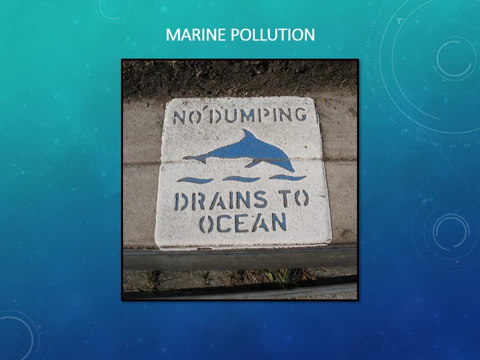 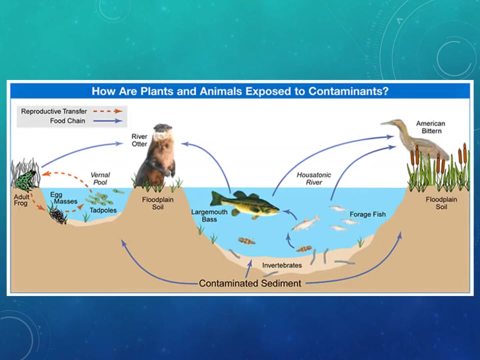 There are six types of marine pollution. I'll discuss Petroleum or oil, sewage, DDT, PCBs, heavy metals such as mercury and trash. Contamination from all pollutants affects the marine ecosystem through a process known as biomagnification, which is illustrated on this slide. 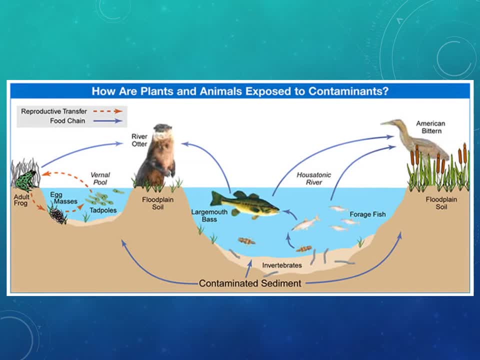 Biomagnification begins when sediments become contaminated and are consumed or absorbed by microscopes. The specimens are then sample tested In the initial stages of contamination, the isotopic organisms such as plankton, algae or bacteria and seawater. These organisms are then consumed by several species until the apex consumer, a large species of fish, for example, is reached. 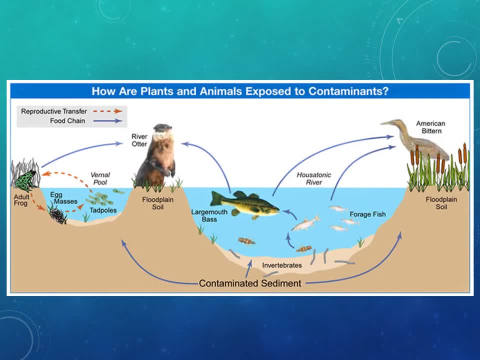 At each phase of consumption, the amount of contamination increases exponentially, so that the apex predator in the food chain has the most contaminants in its body. This means that if we consume fish that are living near contaminated sediments, we're very likely to also be exposed to pollutants. 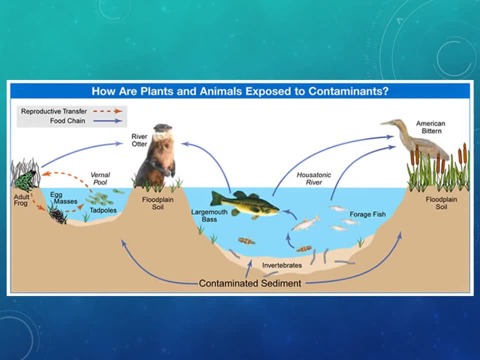 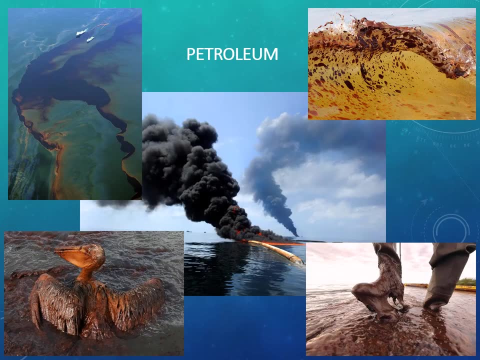 likely to also ingest the contaminants and get sick or, in rare cases, develop cancer or die. Petroleum, or oil, is a major contaminant in the oceans. Oil spills like the images shown from the BP oil spill in 2010 off the Gulf of Mexico. 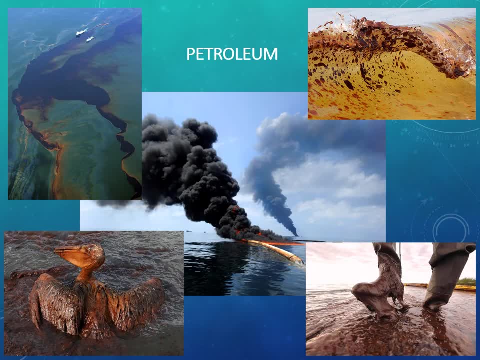 have devastating damage that lasts for centuries, Since oil and water do not mix. again, recalling last week's lecture on water polarity- a surfactant is used to clean the spill. Sewage is also a major contaminant in the oceans. Between 2016 and 2017, the oil spill in the Gulf of Mexico has been a major contaminant. 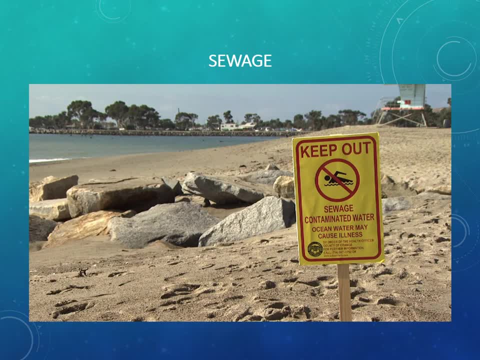 Between 2016 and 2017, the oil spill in the Gulf of Mexico has been a major contaminant in the oceans. Between 2017 and 2018, over 2,000 facilities along California's coast reported sewage spills and over half of those have reached the ocean. 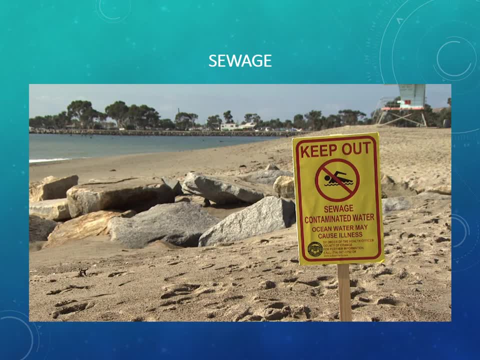 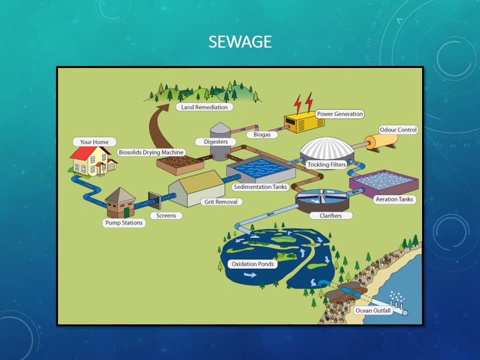 Beaches are often shut down for days to weeks due to cleanup of these spills. Sewage facilities are usually processing plants which recycle or distribute raw sewage that flows in pipes beneath housing, businesses and factories. This diagram shows the flow path of sewage from your home towards the ocean. 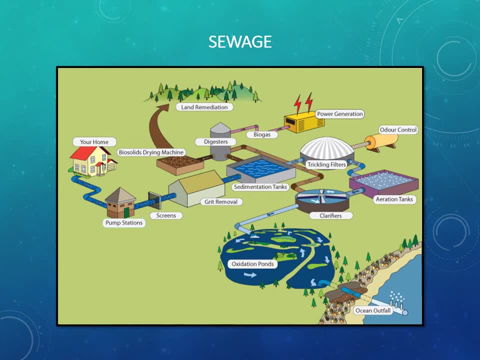 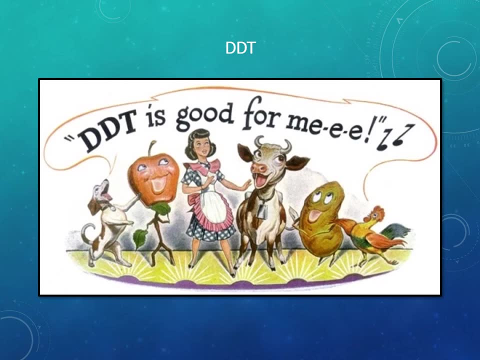 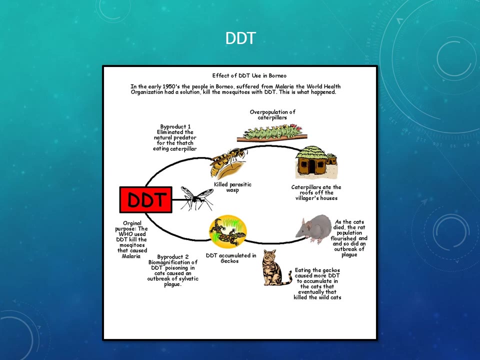 While the next two contaminants have been banned from use in the United States, their impact still affects marine life and ecosystems today. DDT is an organochlorine that was used as a pesticide. It was originally made to combat malaria and typhus spreading mosquitoes in the 1940s, but 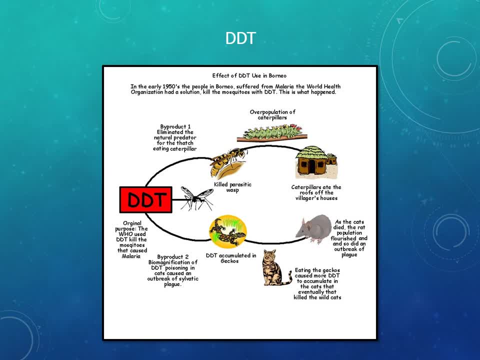 it was discontinued from use in the 1970s due to primarily Rachel Carson's work- Silent Spring. While DDT is an organochlorine, it was originally made to combat malaria and typhus spreading mosquitoes in the 1940s, but it was discontinued from use in the 1970s due to primarily Rachel Carson's work- Silent Spring. 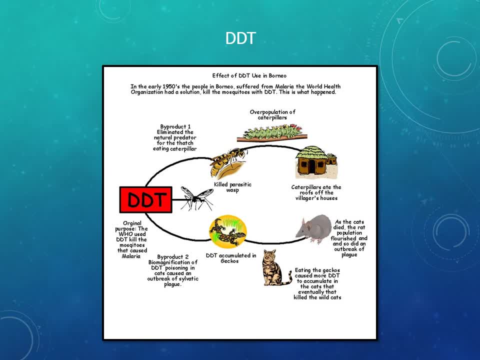 DDT is an organochlorine. it was originally made to combat malaria and typhus spreading mosquitoes in the 1970s. due to primarily Rachel Carson's work, Silent Spring DDT embeds itself in liver and reproductive tissues of birds and other wildlife in wetlands. 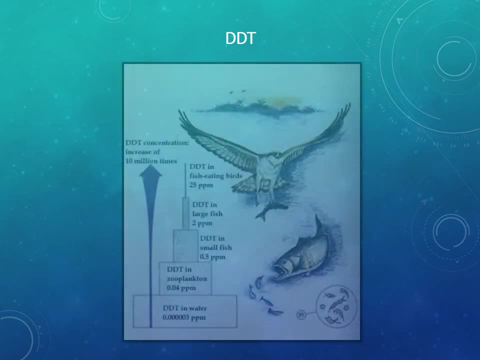 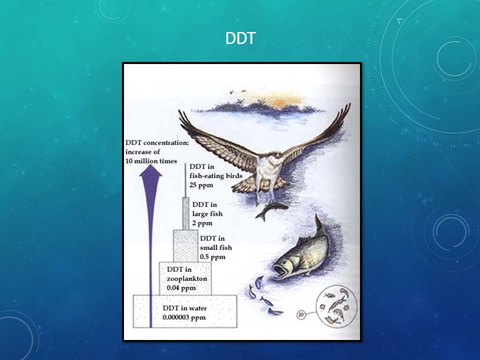 ecosystems. So here's how that process happens with biomagnification. Again, note the parts per million amount in the water. So just a very small amount is all it takes for birds to be affected, So as it embeds itself in the reproductive tissues. 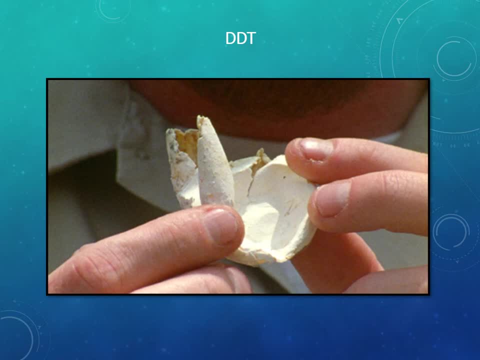 What happens is that birds, essentially when they normally lay eggs, birds have hard shells to their eggs. DDT causes those shells to soften. The calcite that's present in the bloodstream of ovulating birds stops being produced, And so the eggs as they're being laid are very soft. 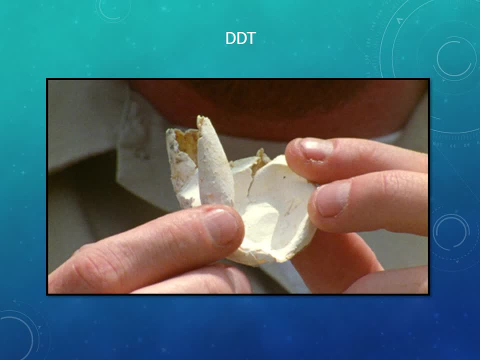 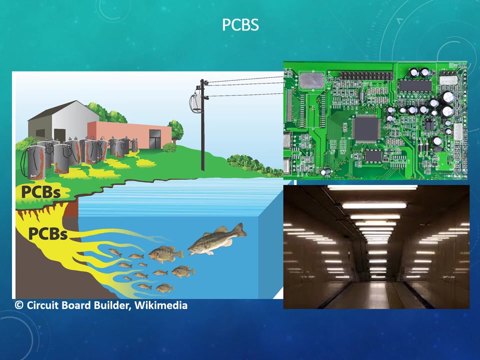 And so the offspring can't survive the hatching process and they die Brown pelicans and other predatory birds along our coast- they almost would extinct due to the presence of DDT. PCBs are organochlorines that are used in electronics, such as microchips, carbonous copy paper and fluorescent tubes. 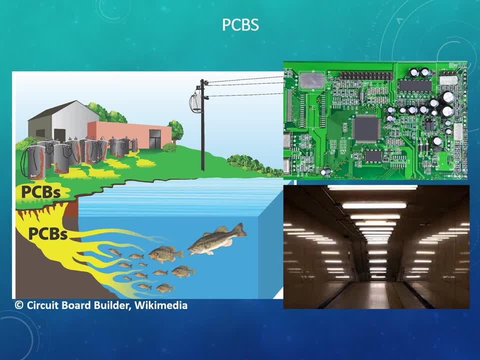 The use of these has been banned since the 70s, but PCBs are still present in sediments from runoff in their factories And have, again, through the process of biomagnification, still been found in various species of fish today, especially in parts of the Hudson River. 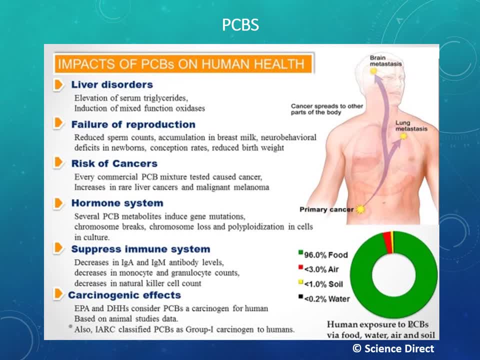 Conception of PCBs is very toxic to us, including children, and especially children, and can lead to developmental disabilities, cancer and, again in rare cases, death. This is just some of the impacts of PCBs on our health, And you'll note that about 96% of it comes from our food, again specifically fish. 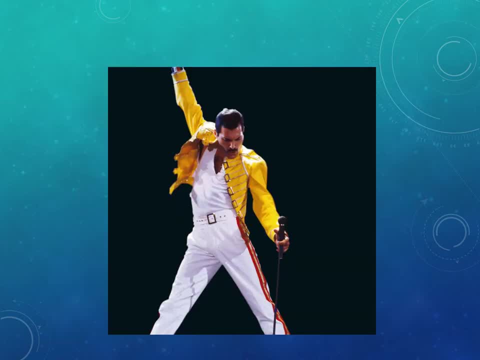 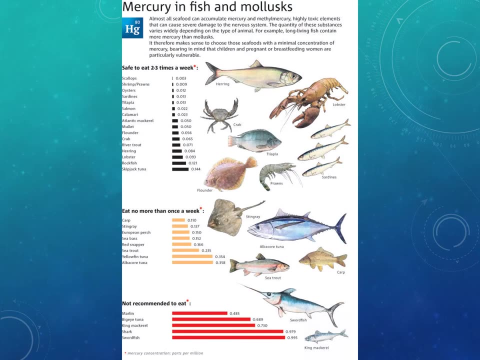 Next, let's discuss mercury. I don't mean this kind of mercury, unfortunately. I mean this type of mercury. Mercury in fish and crustaceans, like PCBs and DDT, spreads through that process of biomagnification. Now, mercury isn't the only heavy metal that we have to worry about from sea life. 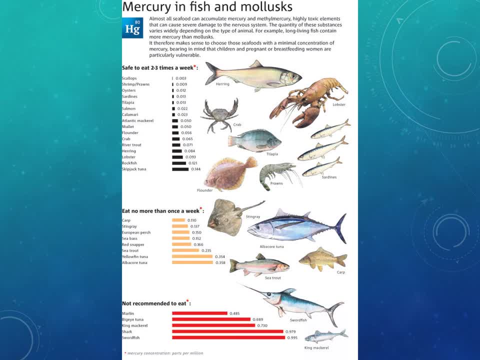 There's also arsenic and lead and cadmium among other metals and other pluripotent metals. There's also arsenic and lead and cadmium among other metals and other pluripotent metals and other pluripotent metals. 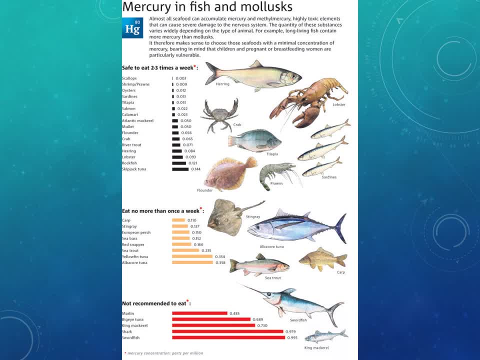 that exist in the sediment, especially where there was toxic waste that's been dumped. We do have to worry about that as well. We do have to worry about that as well. We do have to worry about that as well. So the way that all of those heavier elements are processed is very similar to what happens with DDT and PCBs. 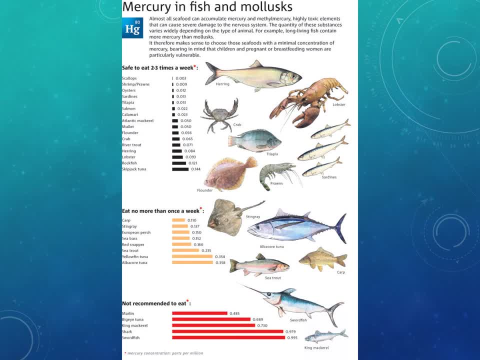 So the way that all of those heavier elements are processed is very similar to what happens with DDT and PCBs. Again, it embeds itself in sediment and different species of plankton and algae consume it or absorb it, And then other organisms eat those en masse. 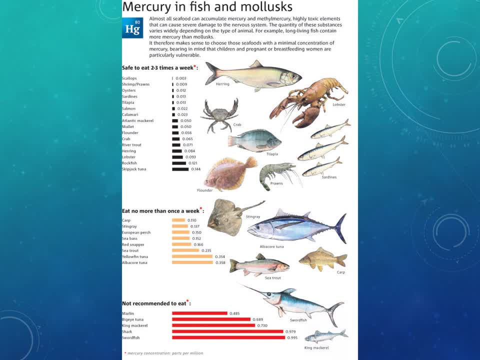 And then in turn, you know, with the food chain, small fish eaten by larger fish, etc. etc. moving all the way up the food chain until we get to these organisms that are listed here. so this chart shows a list of fish that contain certain amounts of mercury contamination and it 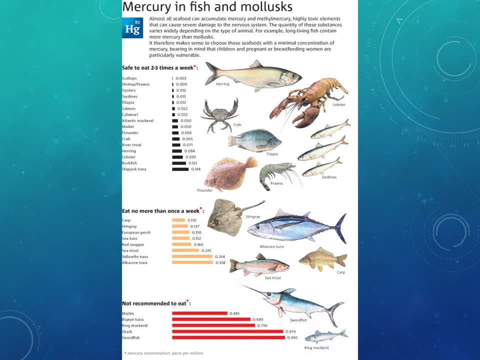 also shows you which fish are safe to eat multiple times a week. so if fish is a main part of your diet, so if you modify your diet to not have as much beef or chicken in it and you prefer to have fish, let's say, for example, you have still have to be very careful about which species of fish that 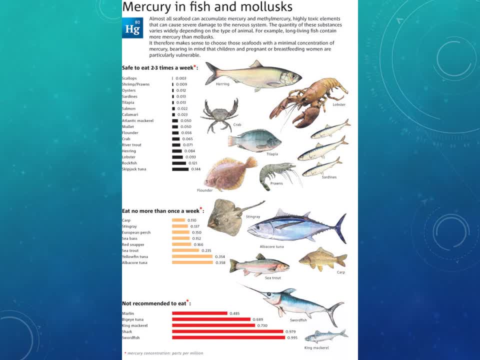 you're consuming and note that the ones that are not recommended to eat include things like sword fish or marlin, mackerel and shark. those species are not recommended because they generally have very high proportions of mercury in their body. mercury poisoning is very serious, as is lead. 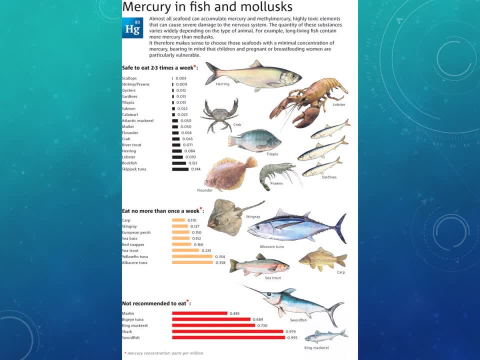 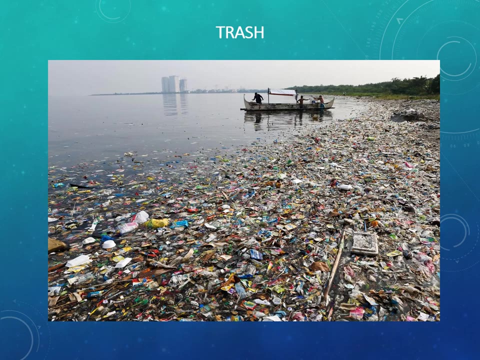 poisoning, it can cause major issues, issues again with not only reproductive tissue but also in your brain tissue as well. finally, the most obvious marine pollutant is trash, and that's something that we encounter every single day. i'm sure most of us don't even really think about it. right, you go to your local. 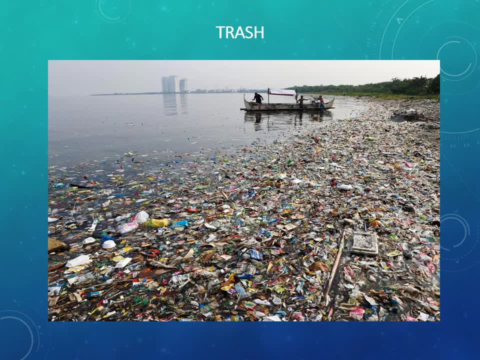 eatery, you order takeout or whatever. you get it delivered to your house and you just throw it away in the trash can and from there you take your trash out to the dumpster. but then most of us don't really think about what happens to your trash after that point. trash that sits in landfills doesn't just stay there. 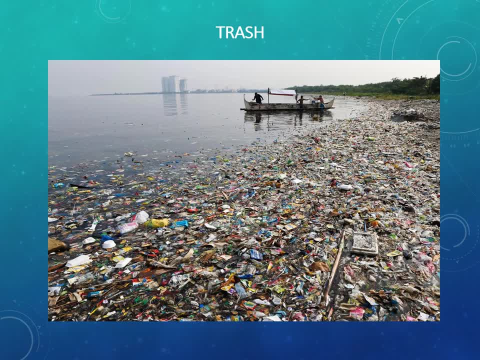 some of it does get compacted and reduced and recycled, but the vast majority of that trash, whether on purpose or whether on accident, becomes some form of litter, and, including trash that sits in these dump sites, you know, for hundreds of years, those materials will eventually end up in the ocean in some way, and so trash is a big problem, not just because it's what we see at. 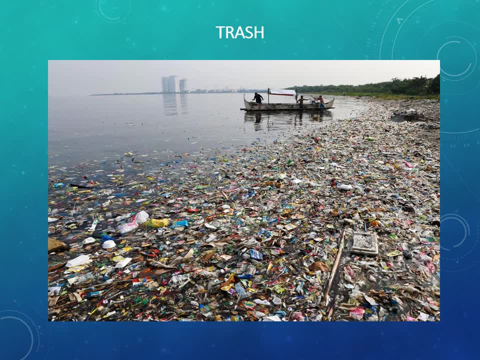 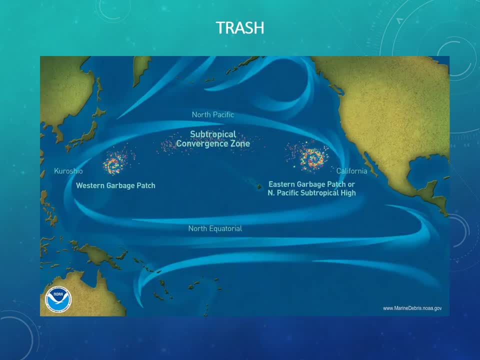 the surface, but it's also because this trash, as it breaks down, just continues to circulate in the ocean for thousands of years. the north pacific gyro system contains a large garbage patch along each major boundary current. that includes the eastern boundary current- our california current- and the western boundary current, the carotio current. now note that these 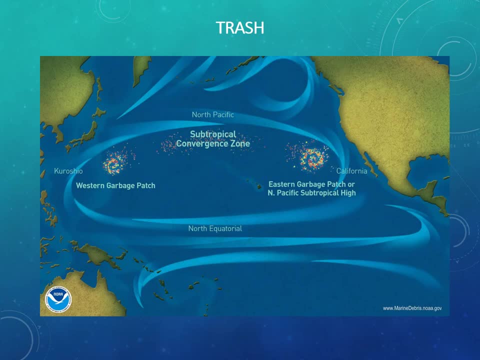 patches are not garbage islands, so i don't know where that misinformation came from, but maybe the state at some point. but instead of like an actual physical island of trash- which i know does exist, but it's not- these patches are not like that. okay, so they're not like a massive pile of garbage. 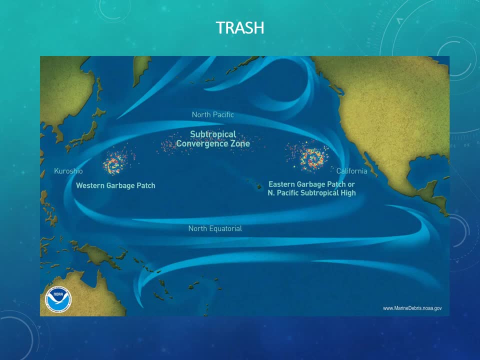 they're actually like. think of them as like soup. so the trash kind of floats around like veggies floating in soup and it drifts with the current, and so the process that circulates- plankton and algae, typically in gyro systems known as eichmann, are transported- also- will pick up our trash and it will move it around and around in this cycle. 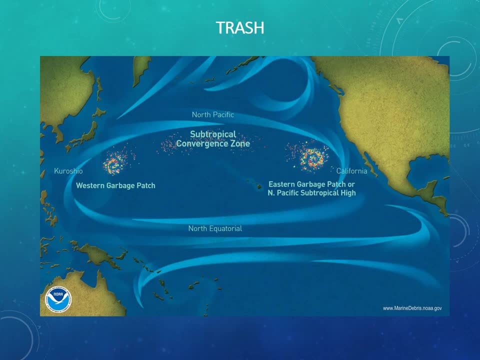 across the pacific ocean basin and, unfortunately, all of the major gyro systems of the world have these garbage patches within them, and every single year, more of this trash is found in the bodies of various sea life. seabirds, turtles and other marine life can not only 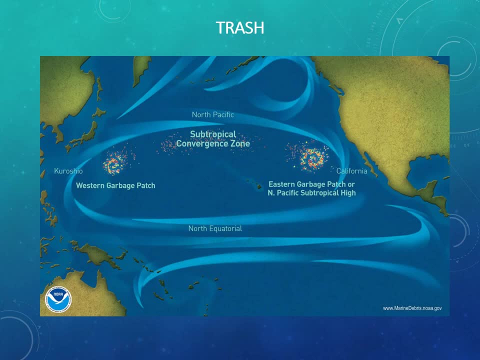 get caught in this trash and be suffocated, but they can also accidentally consume it, and that's what we have to worry about, especially the smaller bits of trash and particles known as microplastics- and it's really microplastics, that's that's what we have to worry about, because it's. 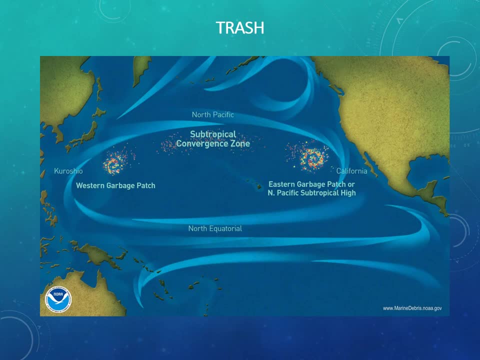 those that do not disappear. remember that the surface of the ocean, as it evaporates, whatever that's floating in the surface waters gets evaporated right along with it, and if these plastics are small enough on the microscopic scale, they can actually be found in rain water and we. 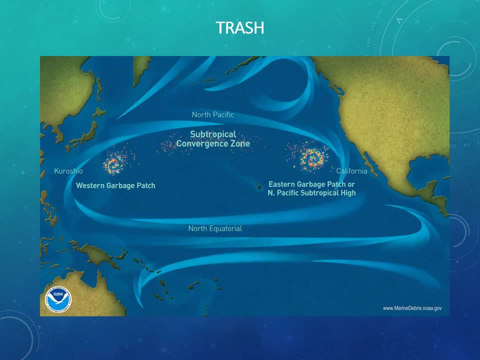 found actually in lake tahoe in california, which was once considered. there's been trash that's found there- microplastics. so, yeah, it's not just what we actually see at the surface, not just what we encounter and throwing out every day, but it's also the microscopic particles of trash that we have to worry about, those plastics. 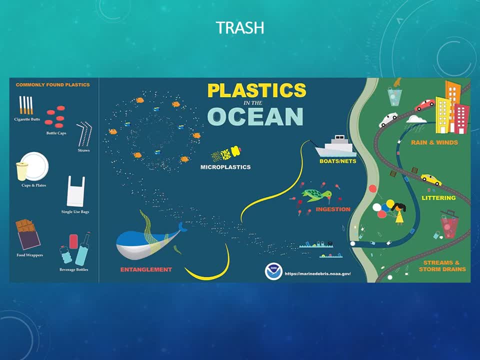 this diagram from the noia shows the common types of plastic that are found in the ocean and what happens as it circulates. in the north pacific gyre most these pieces of trash. they gradually disintegrate into these microplastics, so this is most often a problem with plastic plastics. uh, the reason why it's such a problem. 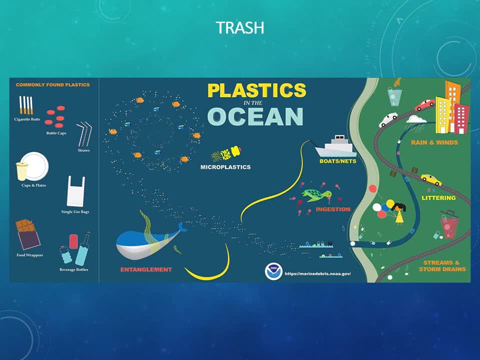 is that? well, first of all, it's very convenient, right? we? we use plastic every day. you use plastic plastics in your phone, plastics in your computer, plastics in your headphones, plastics- uh, you know, in your food plastics and everything that you touch, um pretty much everything that we have. 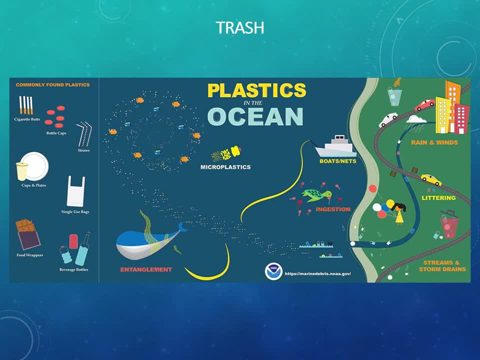 has some form of plastic. uh, all the food containers that we have, elva glass- uh, that's, you know- and the other products we have that are Estados-Union, which are연, water, cling aids, um, um can contain bits of plastic. You know pretty much everything that we encounter in life. 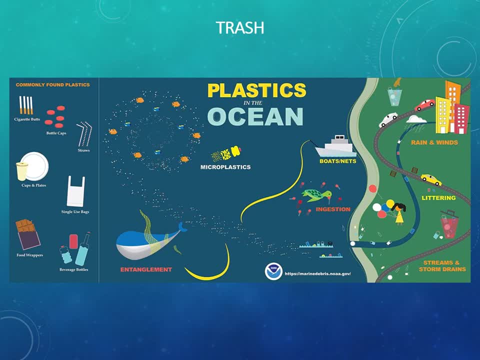 nowadays has plastic in it. The problem with plastic is it doesn't break down, It's not biodegradable, And so that includes plastics in the ocean. So, unfortunately, any debris that we have, whether it's primarily from boats or nets, or whether it's from things as innocuous as 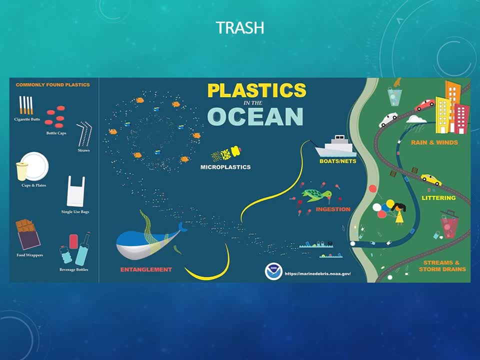 you know food wrappers, these materials. they just float and sit around the drift in the water and they will gradually disintegrate into much smaller microplastics. Again, that's the main issue that we'll have to face: How do we get all the microplastics? 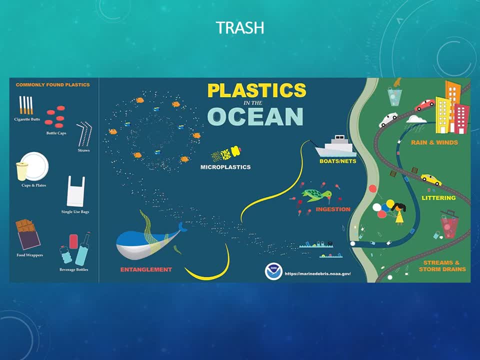 out of the ocean, aside from the large debris that we find, Because, remember that the circulation of the ocean, the remnant time of the ocean, is about a thousand years. So that means that, as these currents are flowing for thousands of years, the trash is filling with it. 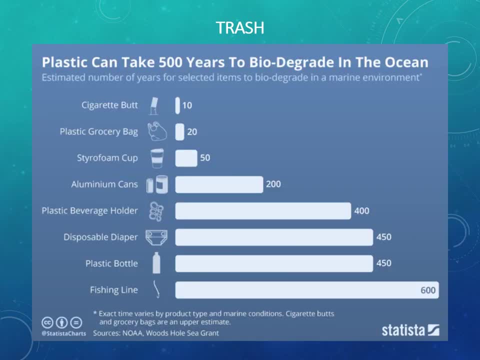 So this diagram shows how long plastics will remain in the ocean. You know if the fishing line lasts the longest, and it's up to 600 years. So again as a comparison, right, A thousand years for water, 600 years. of those thousand years there's like plastic bottle pieces and fishing. 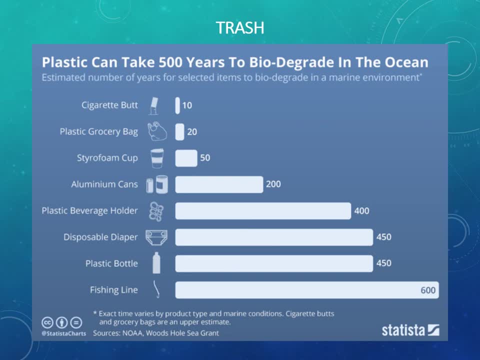 line floating around. So, again, one of the main issues that we have to face is that the ocean is not clean. So the main issues that we'll have to face in the future is: you know, how do we clean the ocean, How do we maintain our oceans for future generations? And we are 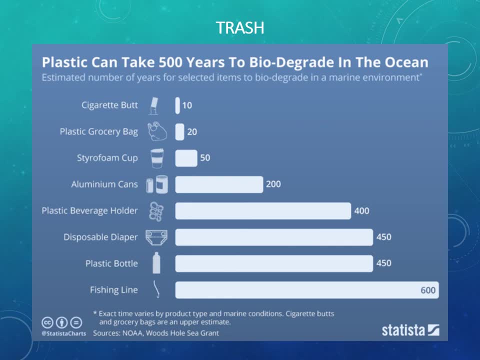 starting to come up with solutions. There are various species of fungi that are being developed right now by laboratories, I think in parts of Japan, where these fungi and algae will start to eat plastics, microplastics. So we are coming up with solutions to this that are natural solutions. 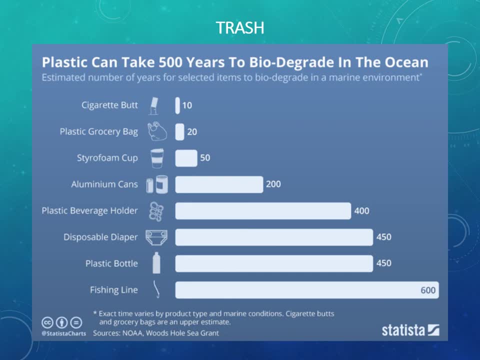 that are helping us to clean the ocean, And we're also starting to come up with solutions to this that are helpful to the environment. potentially maybe, But how we choose to also control our emissions of carbon dioxide and methane gas will have an effect on the temperature variability of. 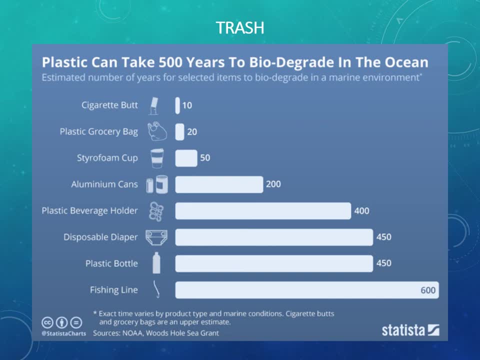 the ocean And without the ocean. keep in mind that without the ocean, we ourselves would not exist. Our species would not be here. Without the ocean and its regulation, we wouldn't have the climates that we do today. So it's vital that in the future,